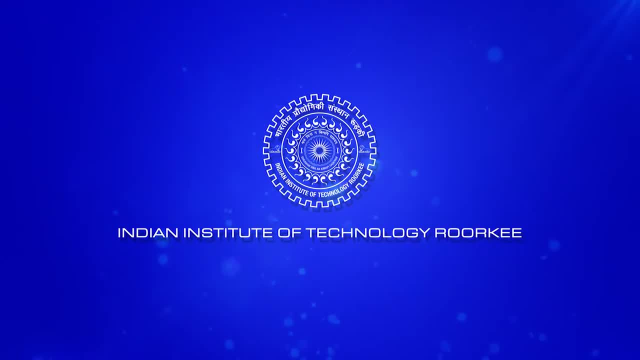 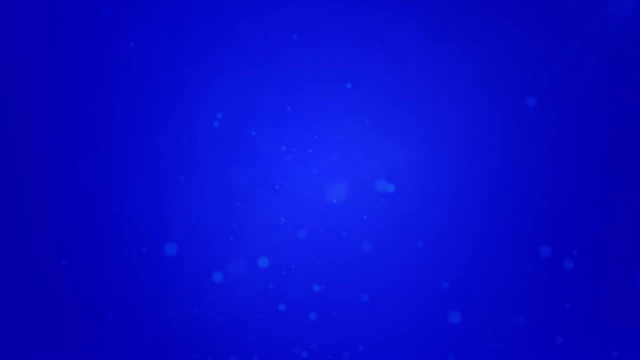 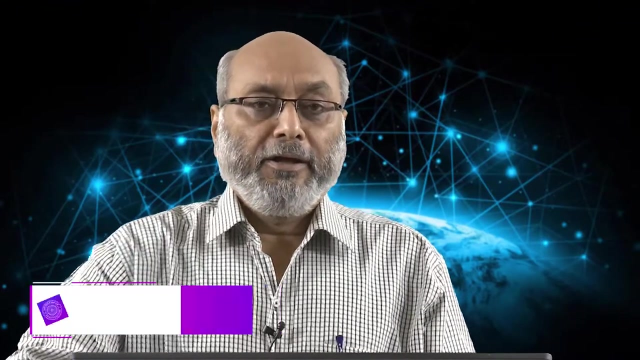 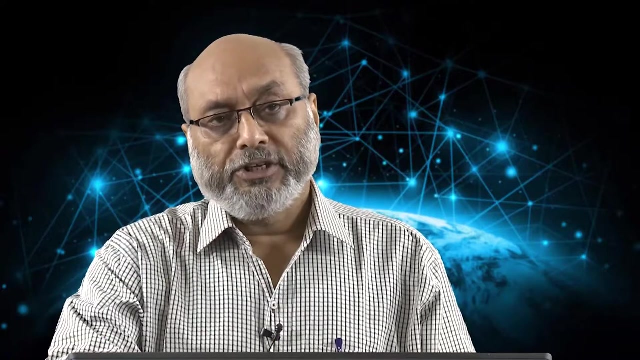 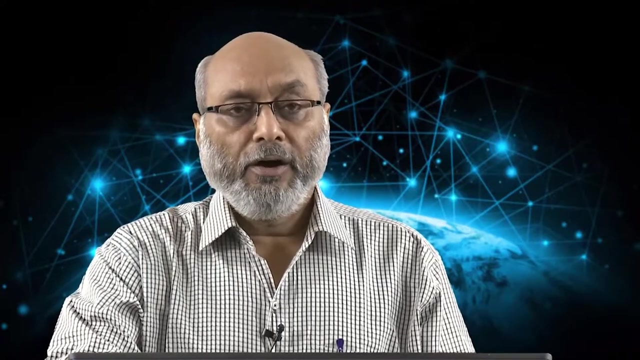 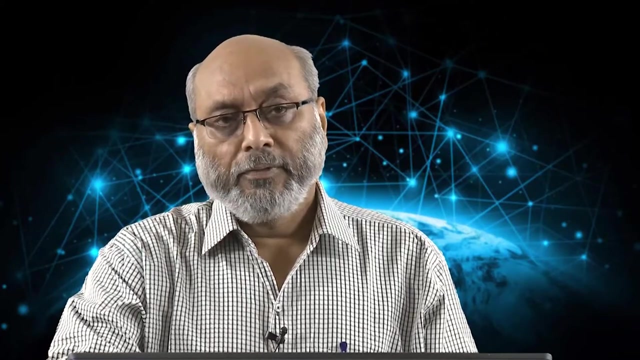 Hello everyone, And today we are going to have a discussion on how to use DEMs For DEM simulations, these DEM for reserve, or we can call as reservoir simulation, and how these DEMs which we simulate can be used in groundwater hydrology, Because nowadays, 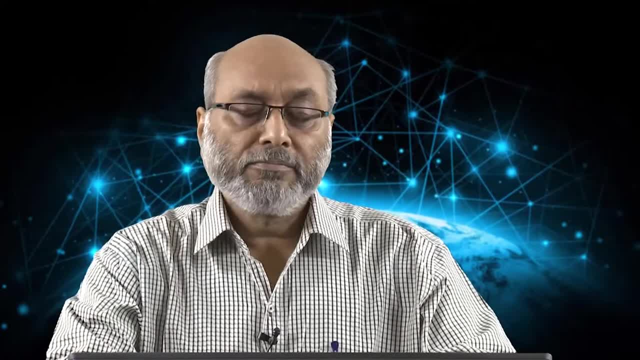 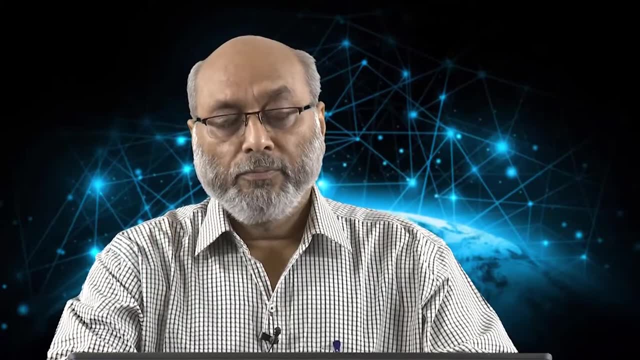 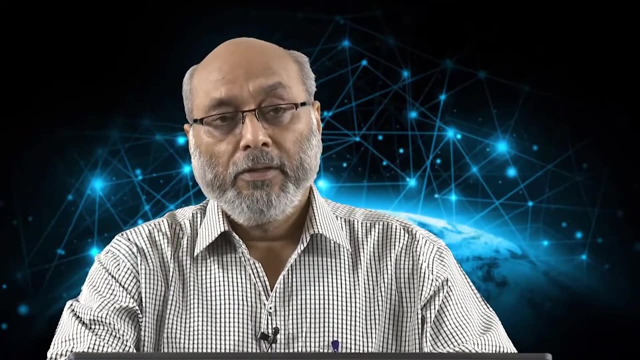 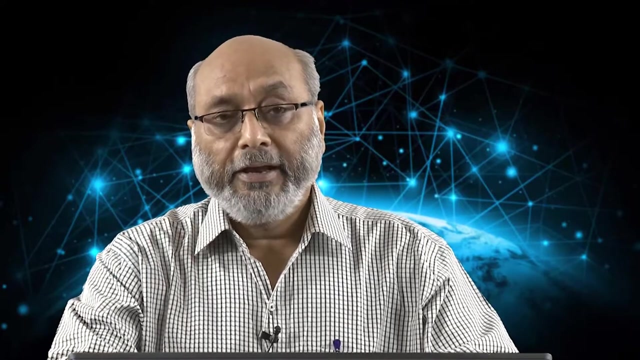 you know that, especially in hard rock part of India, water is a big problem, especially in the summer months, say April, May, June, Even in some areas even in July month. So how to augment groundwater using this rainwater? and that can really. this simulation can help decision makers to make appropriate decisions. 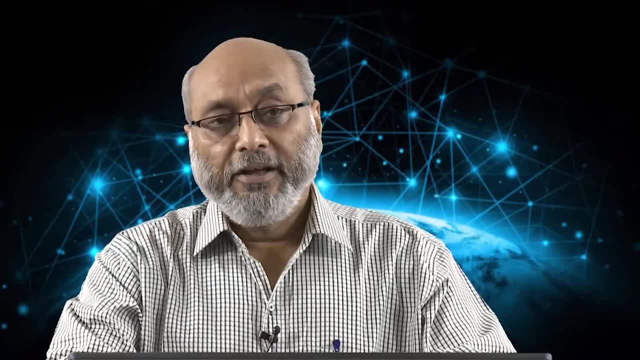 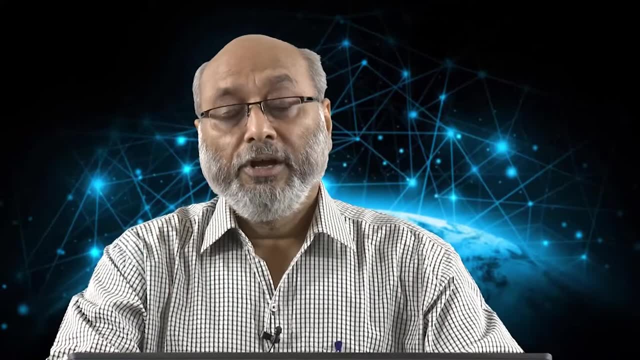 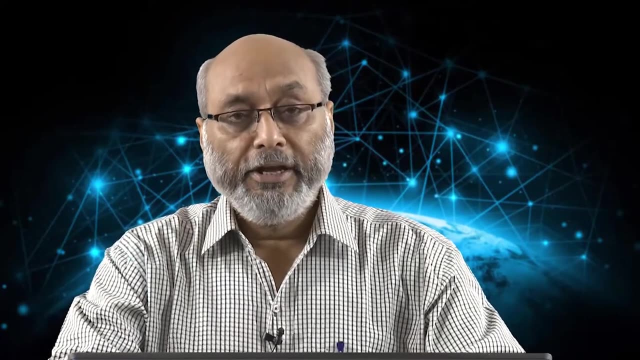 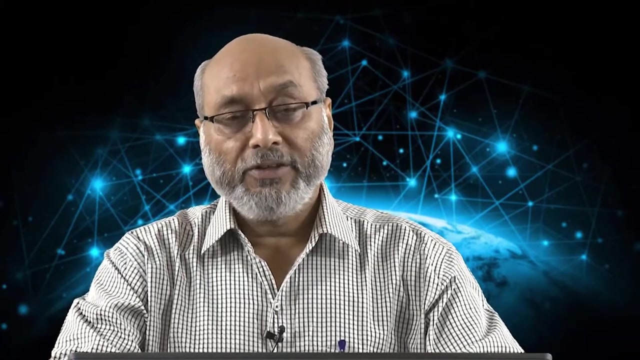 And recently different states have started, you know, some projects just to augment groundwater and also rejuvenation of various streams. Like in Uttarakhand, they are also doing a rejuvenation of Vispana river, which is not perennial ephemeral channel, which passes through Dehradun Also. we understand that 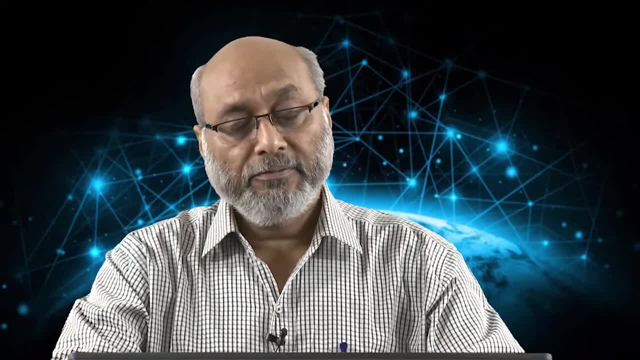 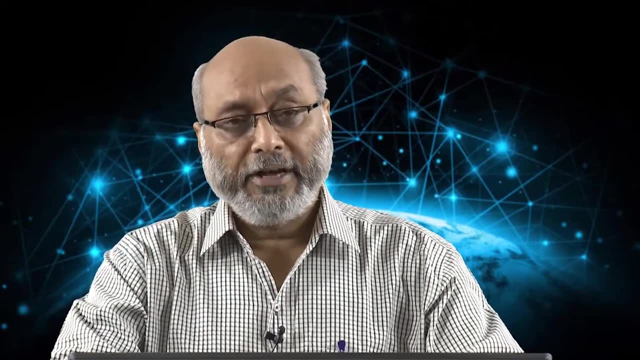 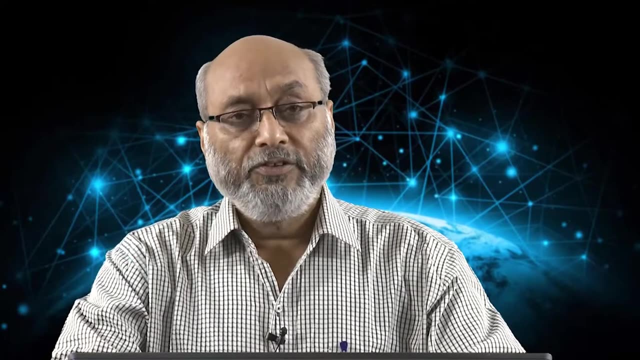 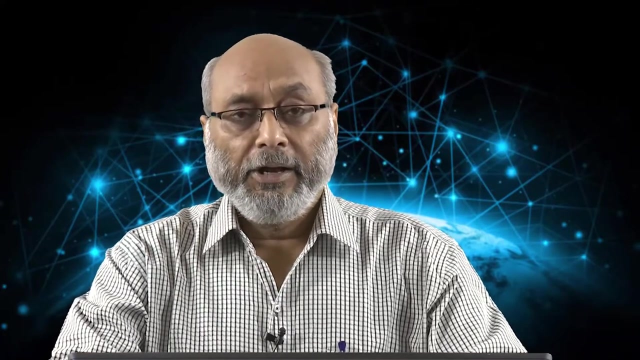 similar kinds of projects are being planned in Andhra Pradesh And in earlier several such projects have been done by some non-government organizations in Rajasthan also. So what is happening? that we are having almost sufficient rainfall or precipitation in total one year, But most of the majority of that water which is coming on the surface of that in form of 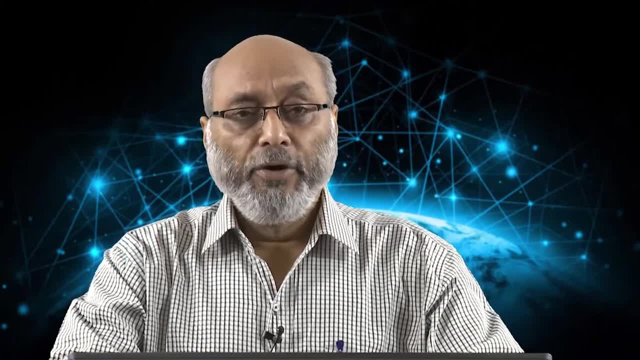 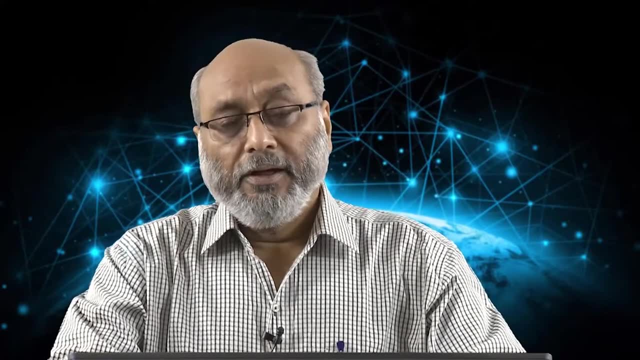 rainfall or precipitation is going as waste, as a surface runoff, into either Arabian Sea or Bay of Gopangal. Now, as you know, there is a lot of work to be done. So what is happening? that we are having almost sufficient rainfall or precipitation in total one year, But most of the majority of that water is going as waste, as a surface runoff into either Arabian Sea or Bay of Gopangal. So what is happening? that we are having almost sufficient rainfall or precipitation is going as waste as a surface runoff into either Arabian Sea or Bay of Gopangal. Say, for example, about 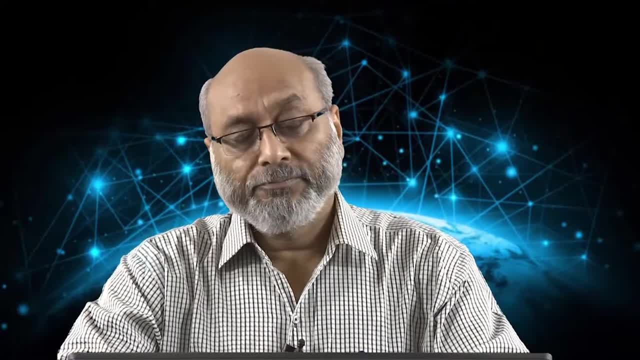 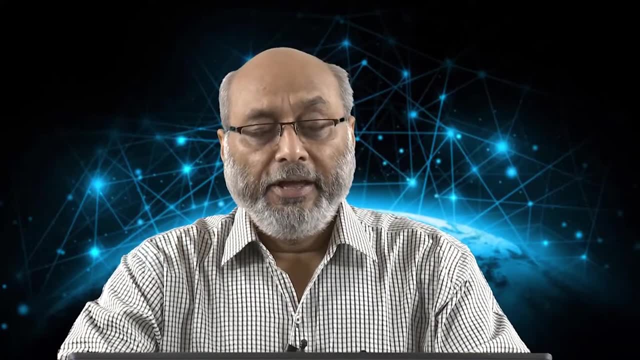 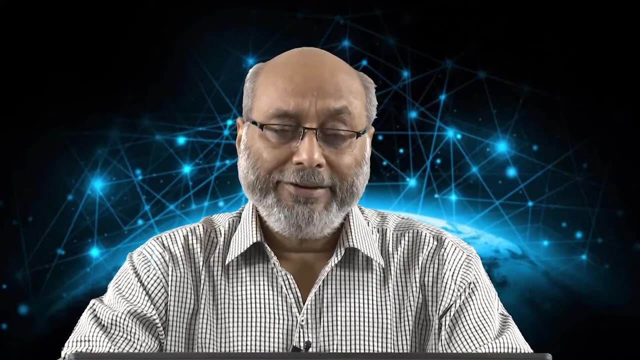 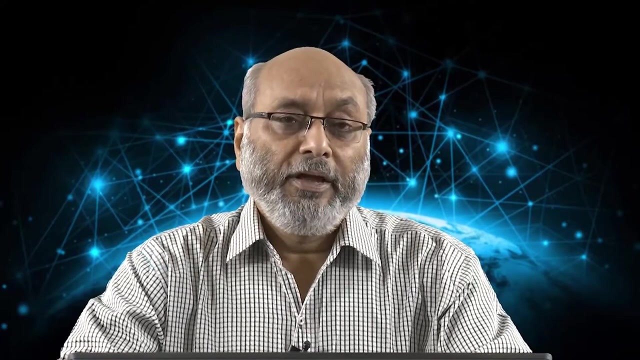 roughly 95% of total water is going as a waste. So if we start just recharging our groundwater regimes using this water, maybe of 1 or 2%, then I am sure, at least for a decade, we should be able to solve the water supply problem in the country. And this application is quite 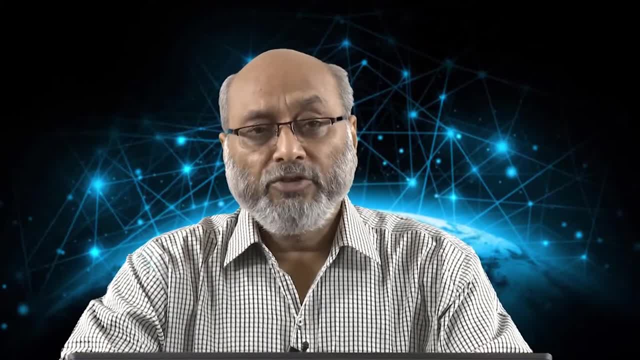 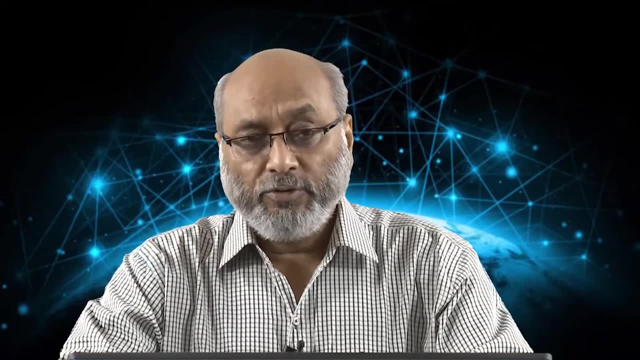 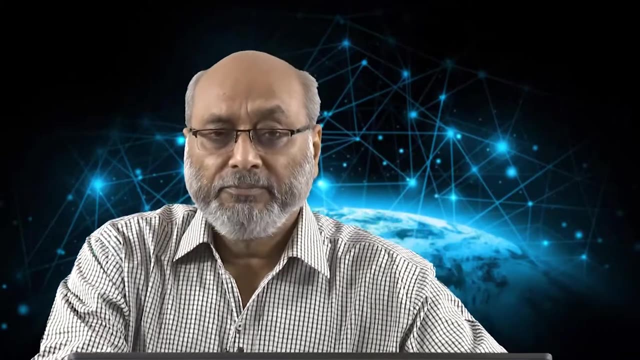 effective of DEMs and the DEM simulations will really help. So this is what we are going to discuss, the application part as well. This DEM simulation we have seen through a demonstration also, But very briefly I will touch here and then we will discuss about this ground As you. 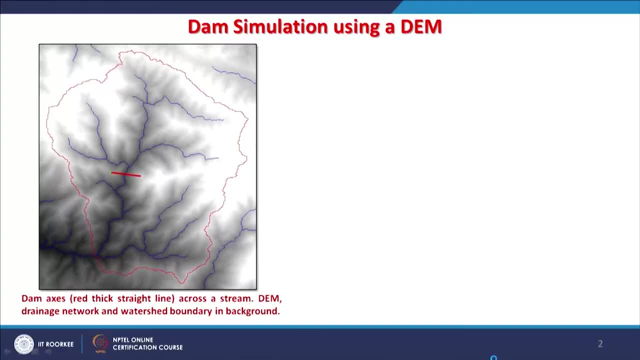 will see that the main input in DEM simulation is a digital elevation model. That topographic surface will help us to find out various options or various scenarios along a channel or in a watershed or a basin, For example. here what we are observing? that there is a watershed and in blue colour, the 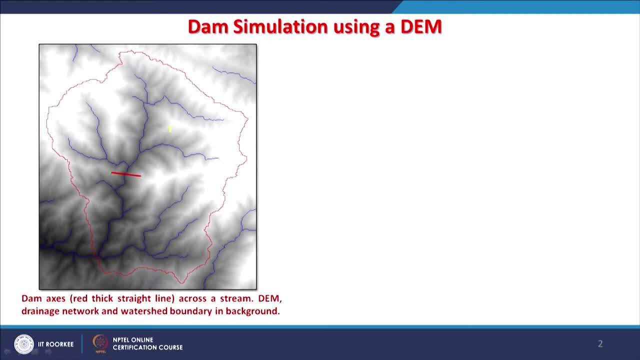 streams are also showing, And these streams have been derived from surface hydrologic modelling. And then a line has been drawn to indicate that here the surface hydrologic dam or a reservoir axis would be there, like of this much length, Now the height of this. 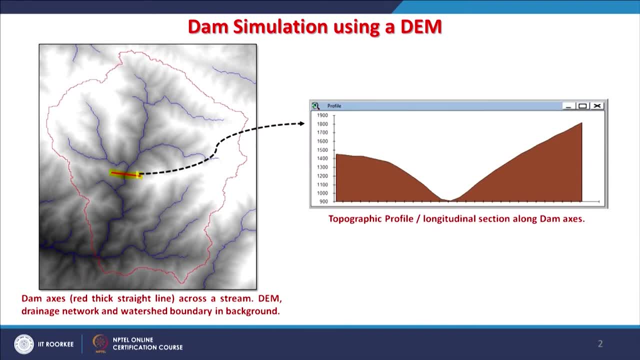 dam axis. we can decide once we start getting this topographic profile. So, like in GIS software, as soon as you draw a line you can get a topographic profile like this. So that means in this part I can fill with water. 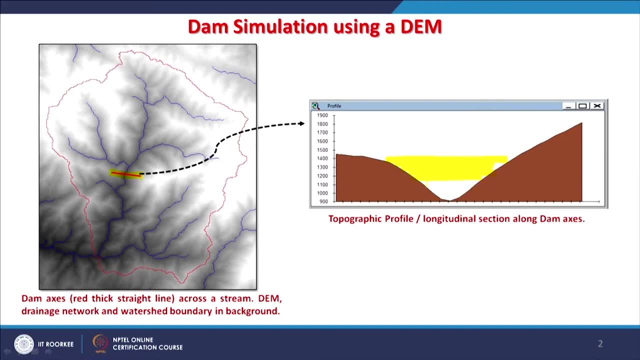 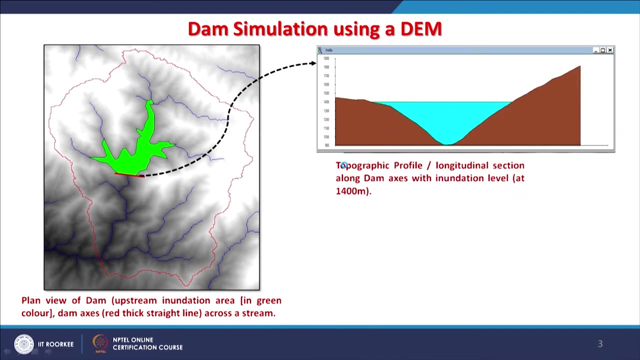 And can create a dam in an upstream or a reservoir in the upstream, inundate the water. So by looking this topographic profile I can fill with water, Like here, this topographic profile once I choose that I want the water level of this meter, that is, 1400 meter in. 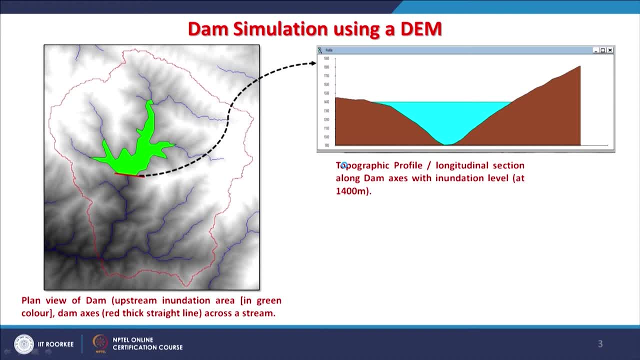 this case this is going to be the inundated area in the upstream. Now reservoir has been simulated very easily. You can also get lot of other datasets like location, length, position and angle of dam. These can also be changes, So if my requirements are not, 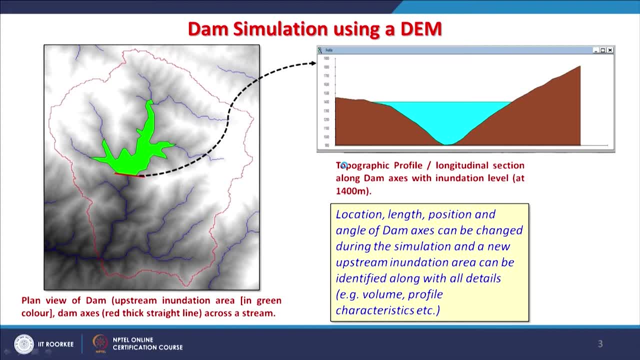 getting fulfilled or I am overestimating or unnecessarily constructing a large reservoir. I can either reduce the height of the reservoir or can go upstream, And if I want more water then probably I can. I can come to this part and can create another reservoir having more storage of water. So 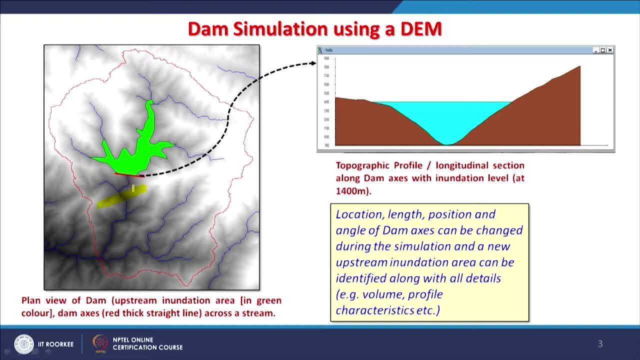 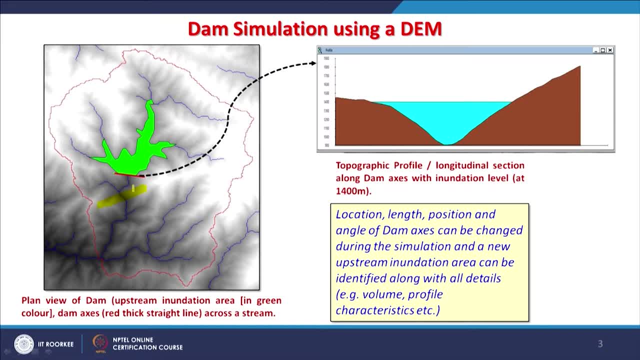 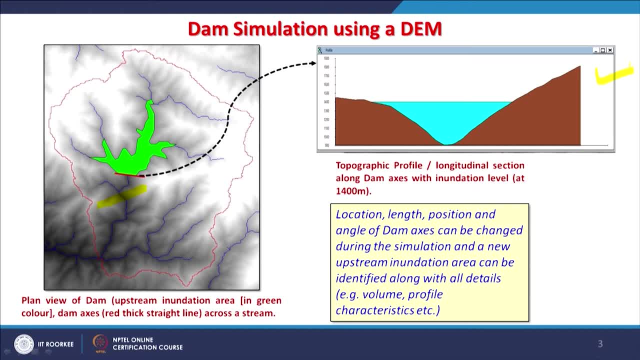 profile, that is the plan and, sorry, the section view or profile view. and here you are seeing the reservoir in a plan, in a 2D. So everything becomes very clear with simple simulations like this. Now, of course, as I have just mentioned you, 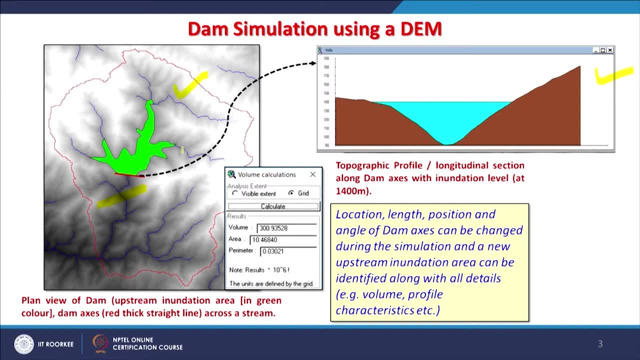 mention that many other parameters which are required to decide or to go for an appropriate decision or optimum decision. then I need what is going to be the volume, what is going to be the area and perimeter of this reservoir. That too can be done. If I do not have GIS or digital elevation model, I tell you with topographic maps it. 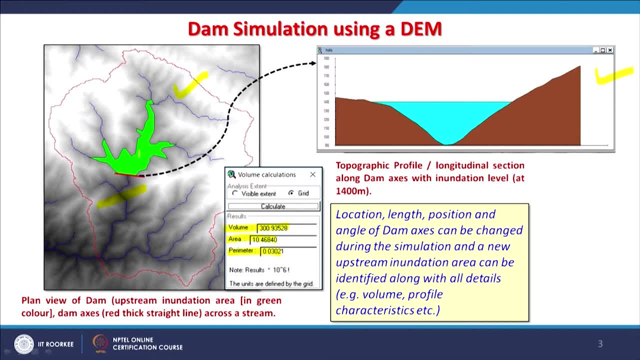 is near impossible to estimate such things very accurately. So what people have been doing? They were using just contour line and deciding based on that reservoir. But if I change the location or rotate my dam axis, then again it has to be calculated. But here, 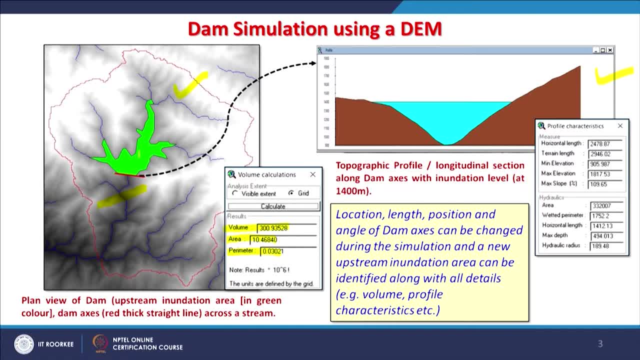 things becomes quite fast and very accurate as well. Now about this profile, the profile which you are seeing, a topographic profile. A lot of many parameters can also be derived here. Important point is, like horizontal distance and terrain length, Horizontal distance is this length which is the top of the water? 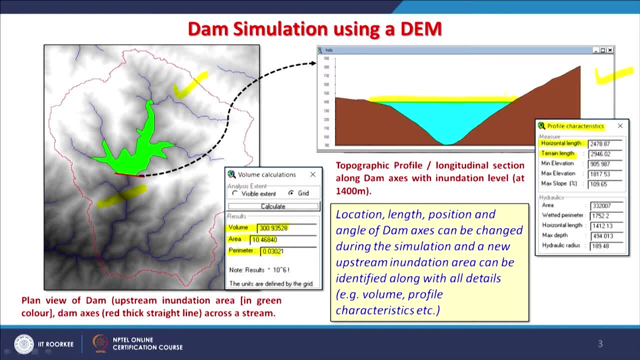 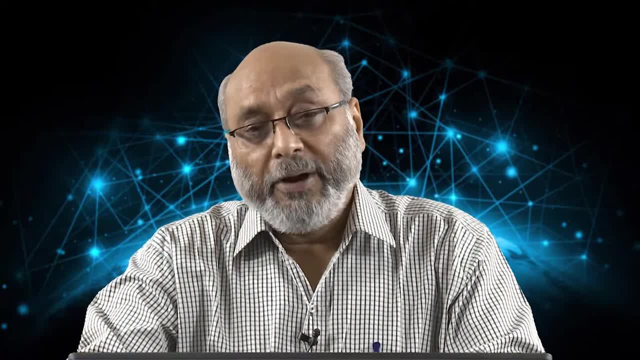 surface. Of course it is in 2D. Recall the discussion when we had about this perimeter, you know, or planimetric length and our terrain length, So similarly here. the horizontal distance and the terrain length, So similarly here. 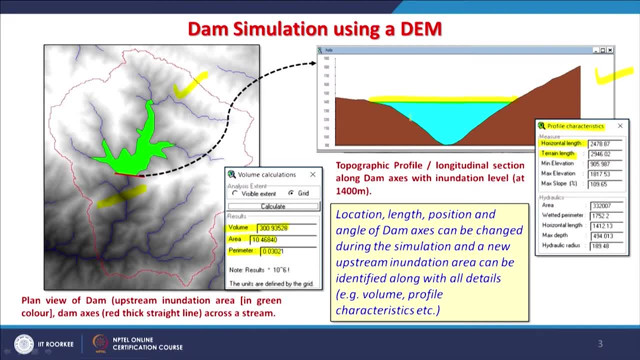 the horizontal distance and the terrain length. So, similarly here, the horizontal distance and the terrain length is the planimetric length and the terrain length is this one, which is this one. So obviously, terrain length will always be more than your perimeter length. 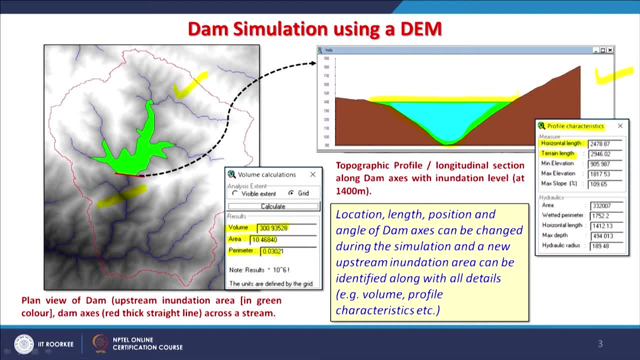 Same would be also with the perimeter. also Now these will have 2 different, like here, wetted perimeter. So wetted perimeter is the part of the water body which will touch the surface or the ground. That is perimeter, Not the perimeter of this polygon which you are seeing on the left image. So this all 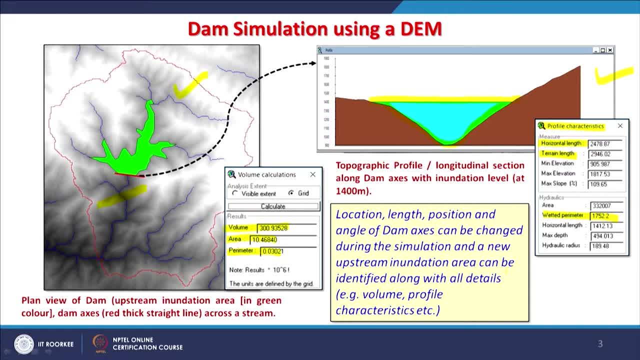 parameters which are required for a civil engineer to decide or design a dam or a reservoir can be extracted from this exercise, that is, dam simulation employing a digital elevation model in a GIS. Similarly, if I change the position, earlier I had like 1400.. If I change, 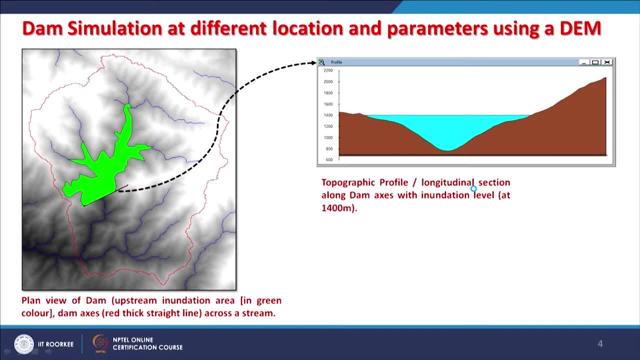 the position earlier, I had like 1400.. Similarly, if I change the position earlier, I had like 1400.. Similarly, if I change the position earlier, I had like 1400.. Similarly, if I change the position earlier, I had like 1400.. Now, what I have done Here: I have shifted the. 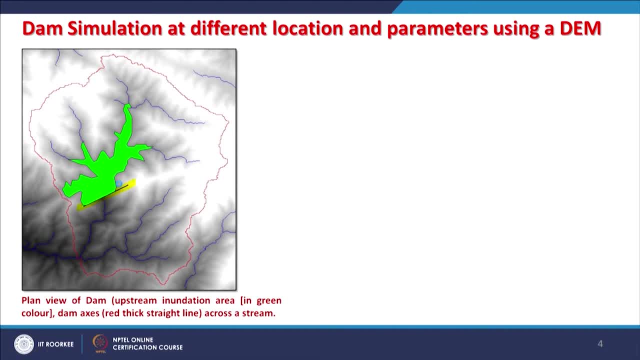 dam axis. In my earlier picture, if you recall, dam was here. Now I have shifted the dam and rotated the dam axis. I am again getting some new values, new locations, everything new. So if, out of these 2 options, which one is better, decisions can be taken before really. anything happens on the ground, And that s the value. If you change the position of the dam, that s the value, So this is what you have done. So, if you have shifted the dam, you have changed the position, And that s the value, So this is what you have done. If you have. 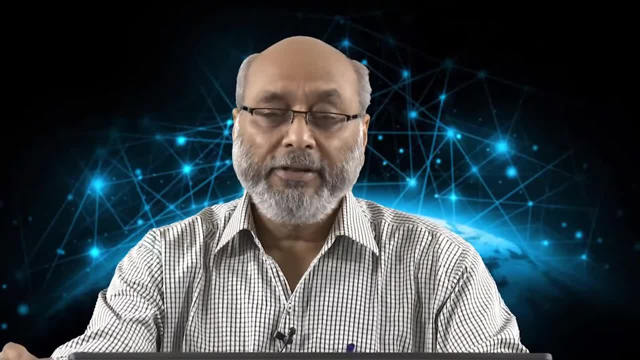 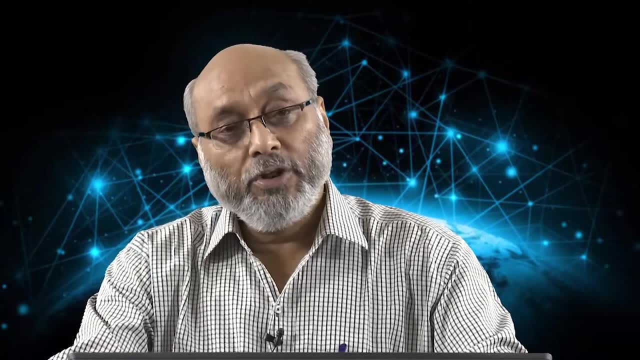 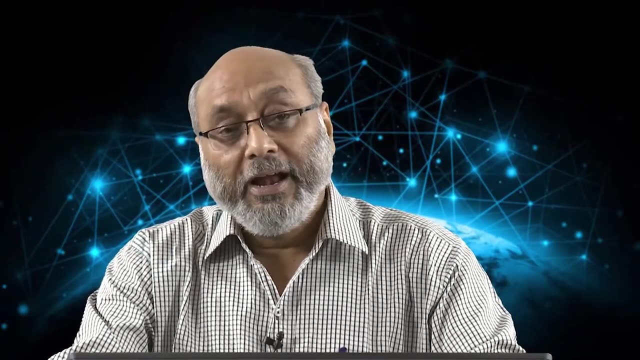 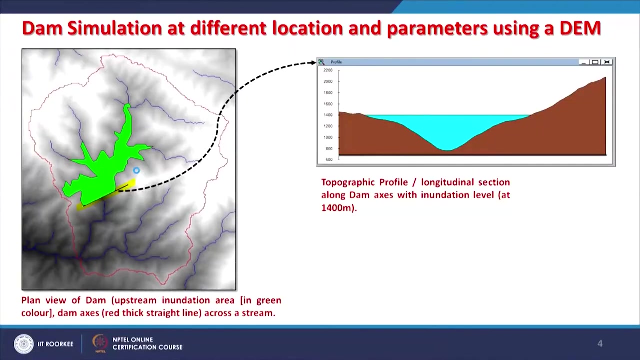 ultimate purpose of GIS, that is, the modelling, Recall, the definition of GIS. What it says, That is say, computer-based information system will store and retrieve, analyze data which is coming from variety of sources and model, as per user-defined specification. So here user is providing all these details: that location of dam, height of the dam. 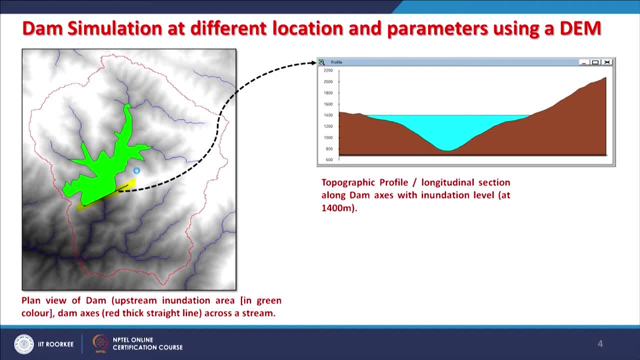 and then the modelling is being done, And ultimate aim of the model is to predict something which has not happened on the ground. but before that, we want to do it. So this is what this platform will allow you And, by this dam simulation, you can do. 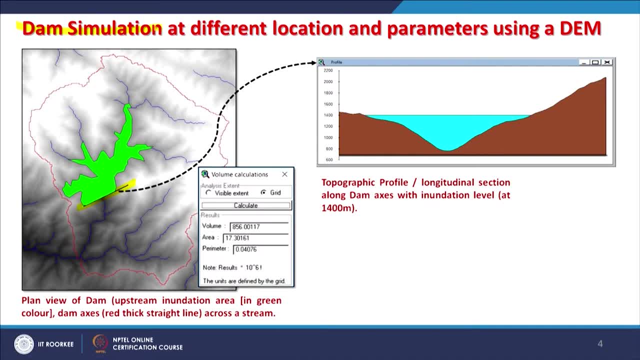 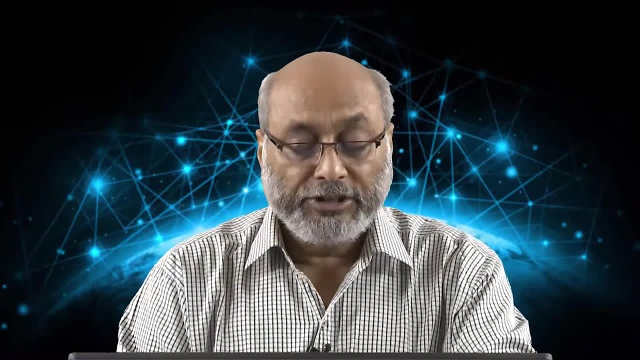 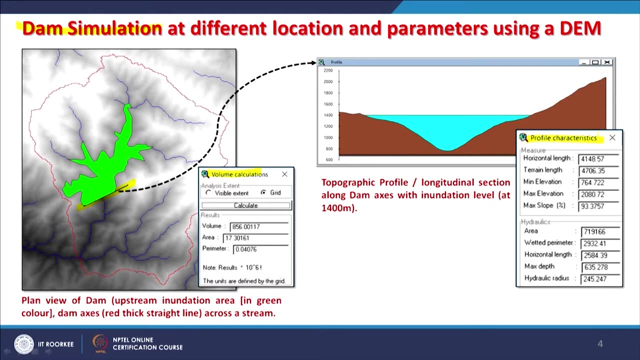 lot of such things. So once I change the location of reservoir height, I have kept the same. Obviously other parameters, that is, the volume calculations or profile characteristics, will also change. Does not matter, I can store as separate. Suppose I had a target of a certain 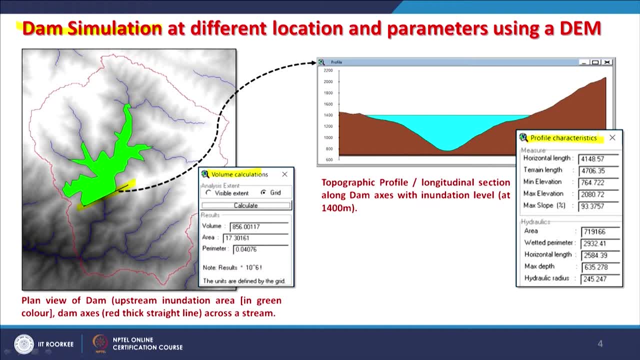 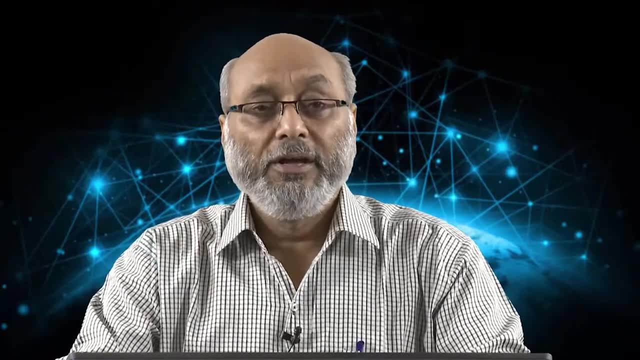 amount of volume of water which I want to store in reservoir. So if I achieve that one, fantastic. If I do not, I will go back again, shift my reservoir maybe to the downstream, Because if you go towards downstream you can store more water, But if I go to upstream, 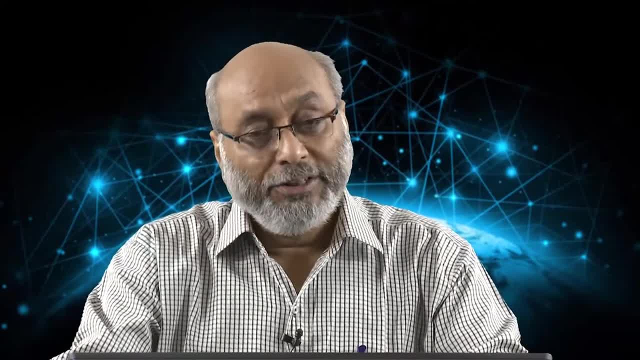 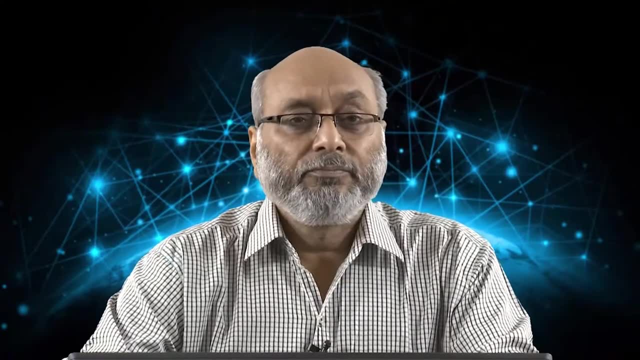 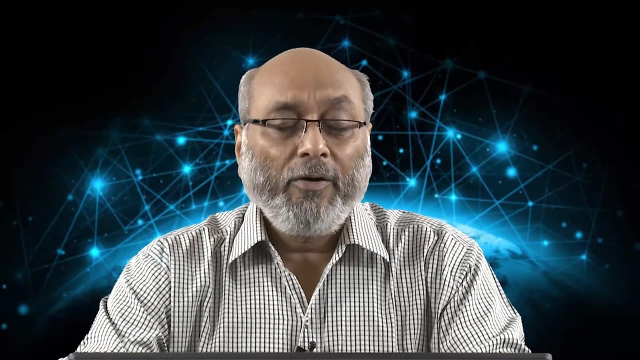 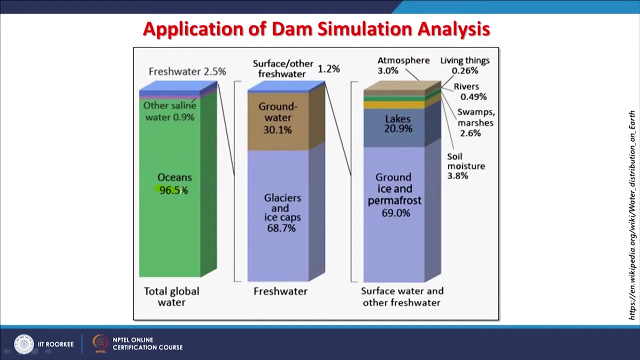 then catchment area will reduce. So that judgment should also be made Now. this is the point which I was just touching in the beginning. The water which we require is very little or part of the total water which is available to us. See, 96.5% of the water is available in ocean. but that is saline. 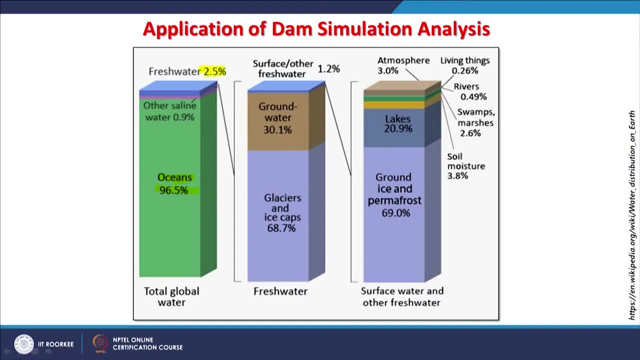 And fresh water is just 2.5%. Out of this 2.5%, 30% is the groundwater which generally we take out and use for drinking, irrigation or whatever- Glaciers and ice caps, which holds about 68% or 69% of total water. And then out of this, of the surface water or the fresh water, 1.2,. this is: 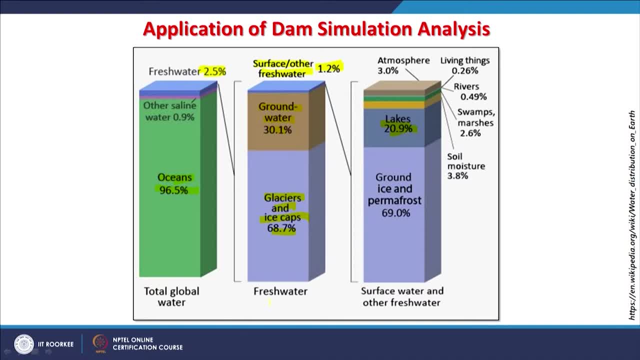 how it is stored. that lakes stores about 21% the ground and ice permafrost about 69%. River water is just 0.49 because most of the water during monsoon time, say in India, is going as a best and does not stay in the river. But of course this is the data for the world. 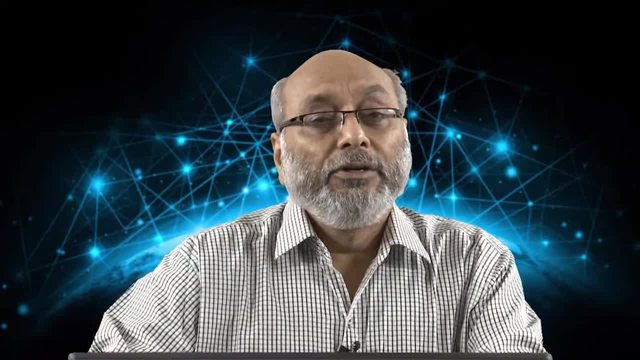 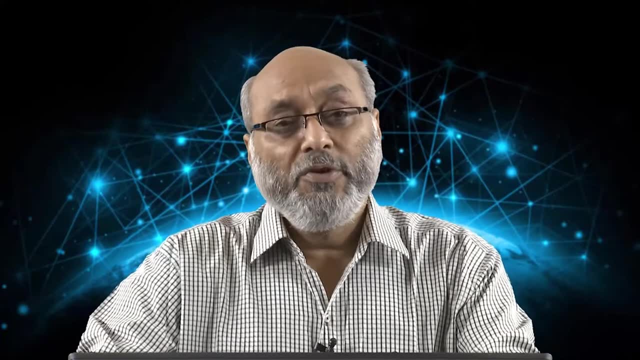 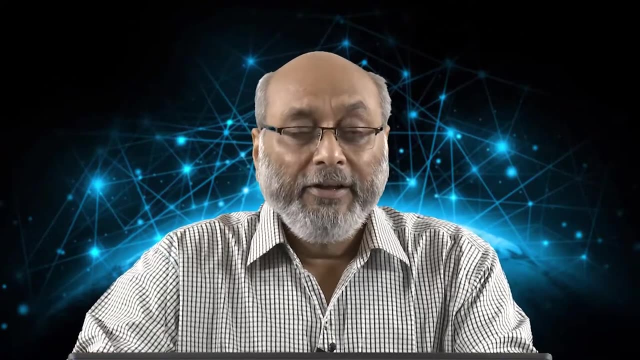 So almost the same scenario in India also. So that means, because the groundwater is an issue, lot of water is going as waste, So we need to store the water, delay the runoff even for a few weeks or months, And if we do it, we can recharge the groundwater regime and you know the groundwater. 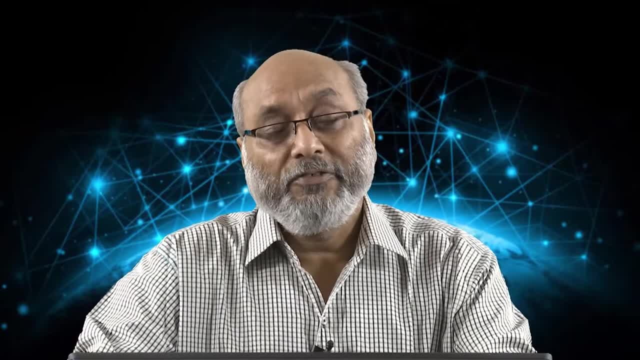 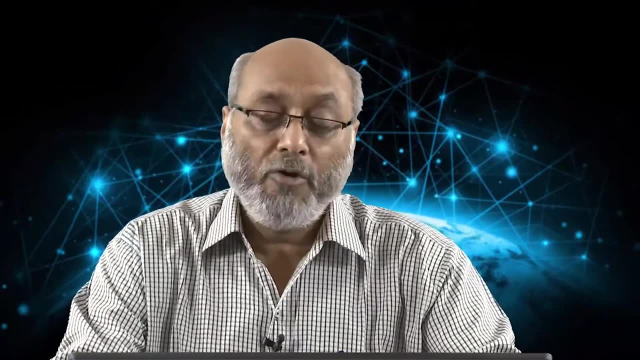 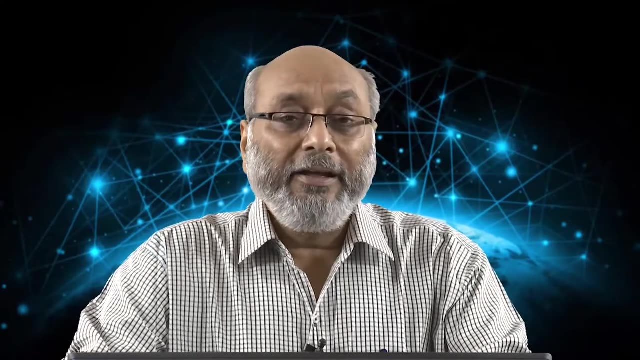 will be available for around the year, rather than surface water, Because surface water there are other issues like loss to the atmosphere in form of evaporation, and can become easily polluted And you know the turbidity and sediments. these are another problems. 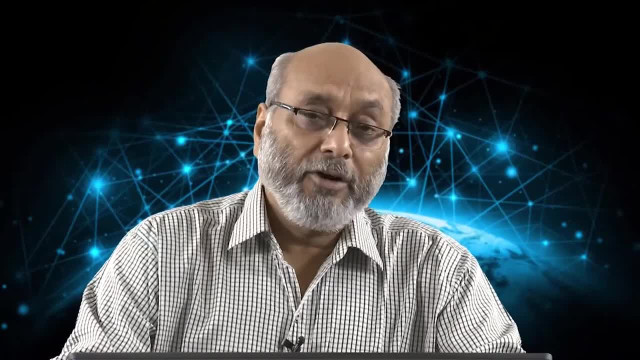 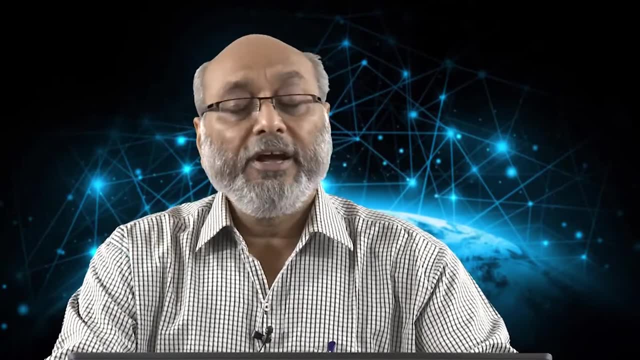 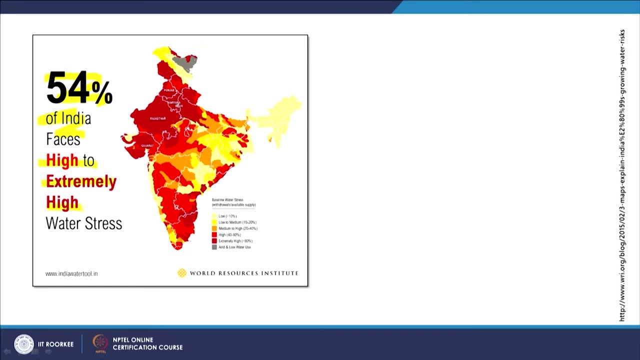 But if we store water in form of surface water only for some time- may not be around the year- then we can solve lot of problems of India in groundwater. Now if we see that 54% of India faces high or extremely high water stress. So, except for north, 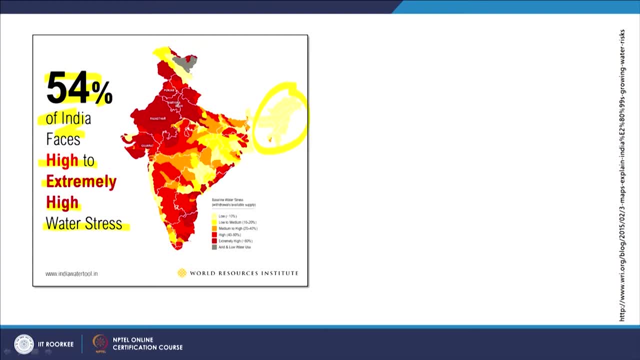 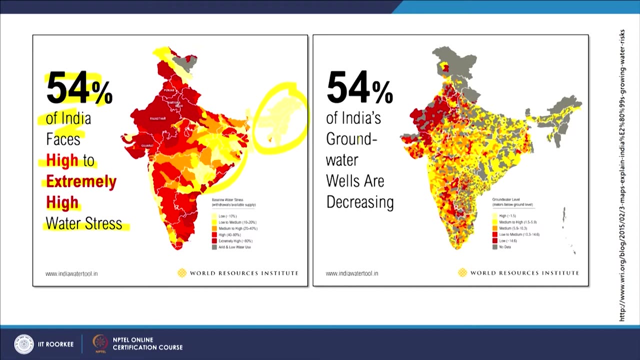 some parts of J&K or some parts of, you know, Andhra Pradesh and Odisha. Remaining parts are really having big-2 problems And if we see that 54% of India s groundwater wells are decreasing, So because we are exploiting more water, Very interesting figure I want. 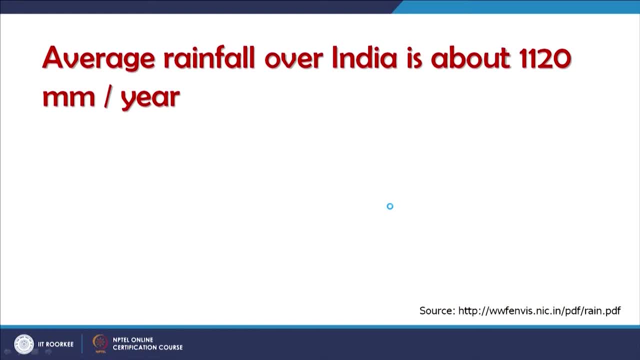 to share with you that the average rainfall over India is about 1120 millimetre per year And if we calculate the total volume of water falling over India in 1 year in form of precipitation, in last 100 years or more it has remained same. That means the rainfall which is or. 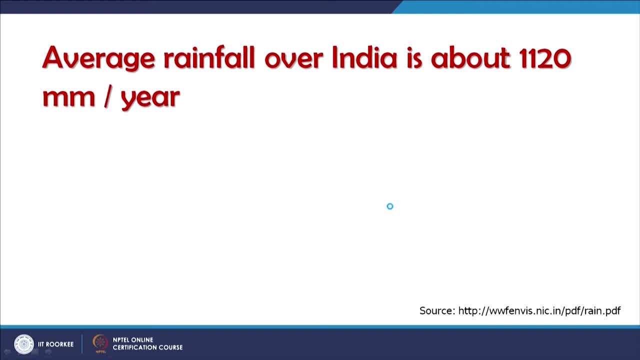 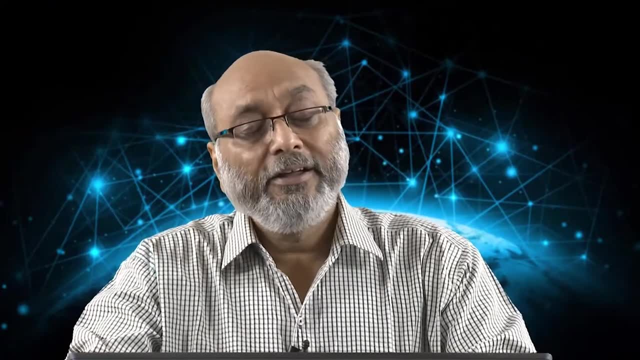 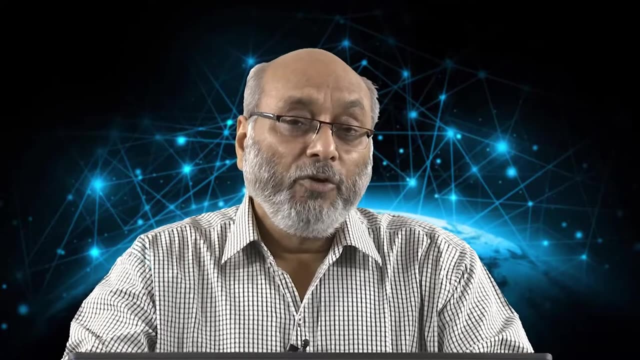 precipitation, which have been occurring 100 years back. it is almost same. The only difference between the rainfall and the precipitation is that the rainfall is increasing. The only thing at that time we had the population of 35 crores like, and now we are having 135 crores. At the time of independence that was the situation. So 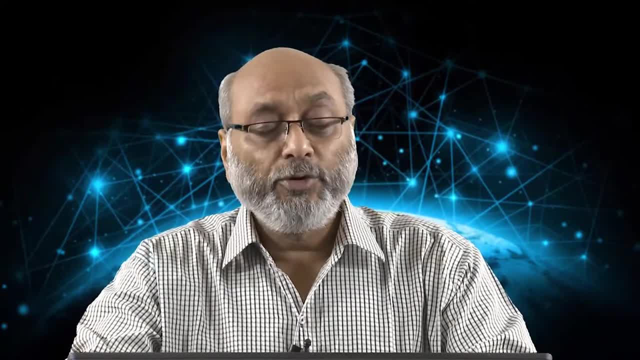 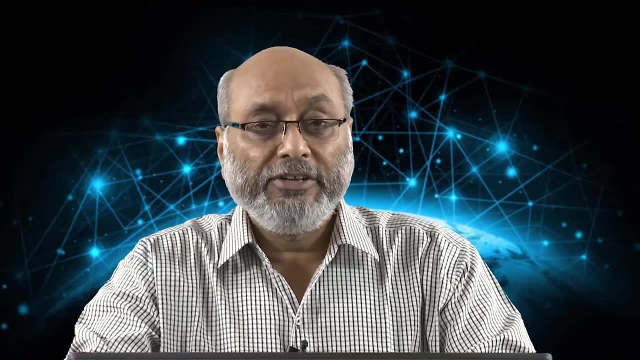 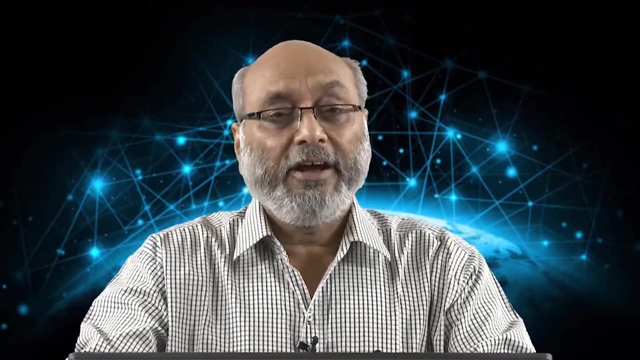 from 35 crores from 1947 in 2020, we are having 135 crores, But the augmentation, rainfall input has not changed, Only the output over exploitation of water And that problem, as I have been saying further. I will add: 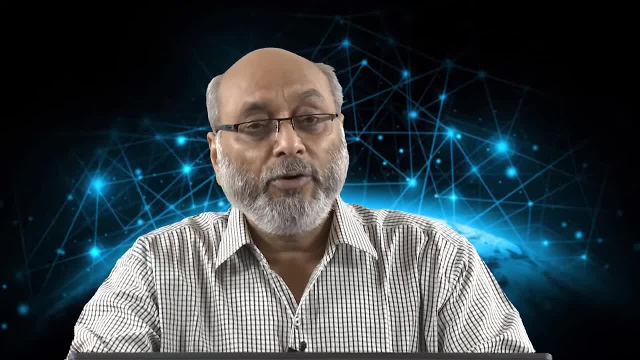 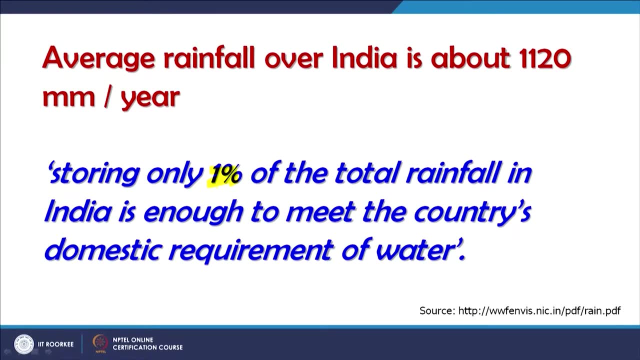 That this problem can be solved in 1 or 2 years time. If we start storing even 1% of extra water of rainfall for the domestic requirements, at least drinking water problem can be solved. But if we add 2 or 3% of total rainfall goes in groundwater, then irrigation and industrial 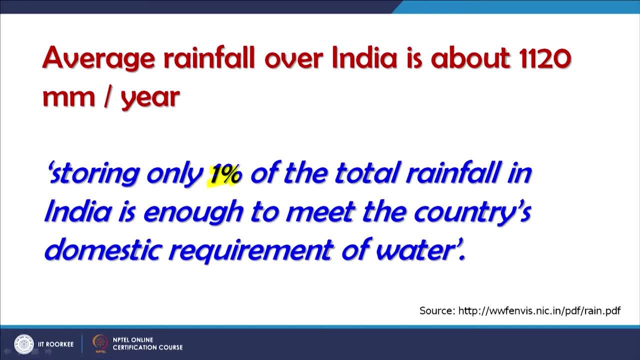 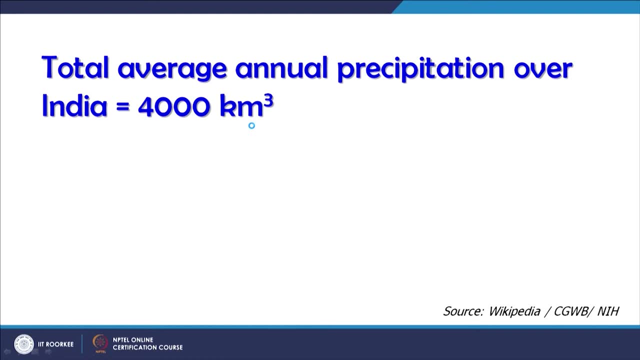 requirements can also be solved, at least for a decade or so. But if population keep rising like this, then we have to create this. one may be 10% of total rainfall Rather than just 2-3%. So now that average annual precipitation over India, which 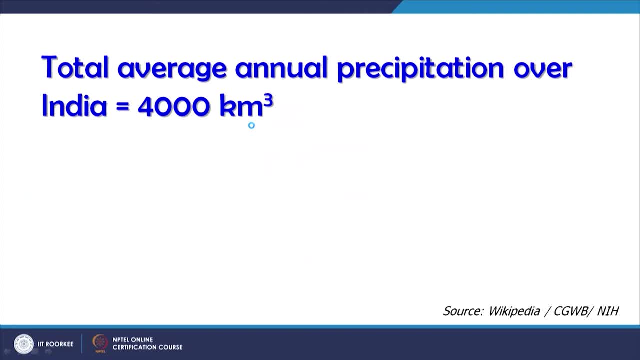 I was mentioning, have remained constant, almost constant, in last more than 100 years, which is about 4000 cubic kilometres total, Wow. And groundwater recharge is just 433 cubic kilometer and rest is going as a based. You are having surface runoff. maximum part is going as surface runoff. It does not store. 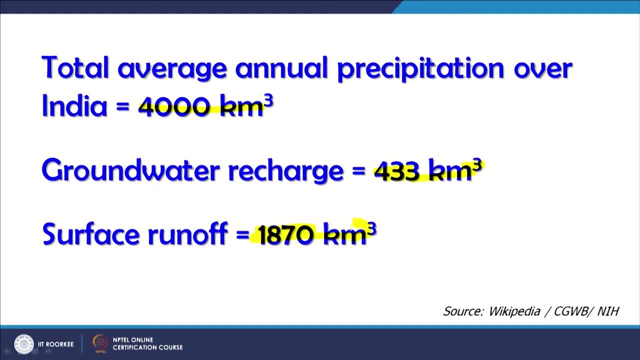 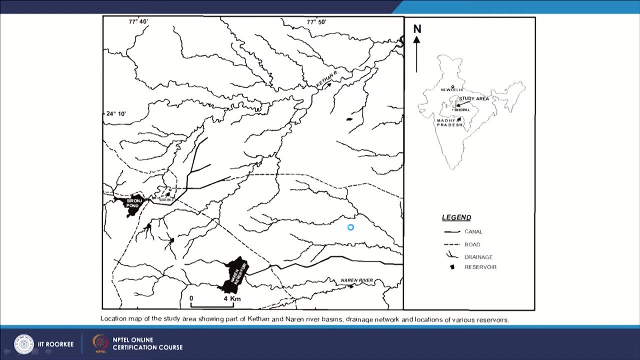 Now I will give you this all idea how to do it, how to solve this problem, through a case history or a study which we did few years back. If you see in this figure, you would find that there are 3 or 4 reservoirs. 2 are big, 2 are very tiny, relatively. One is here, Naren Reservoir, Another. 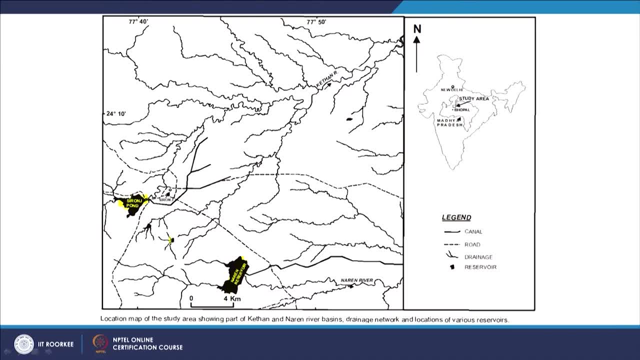 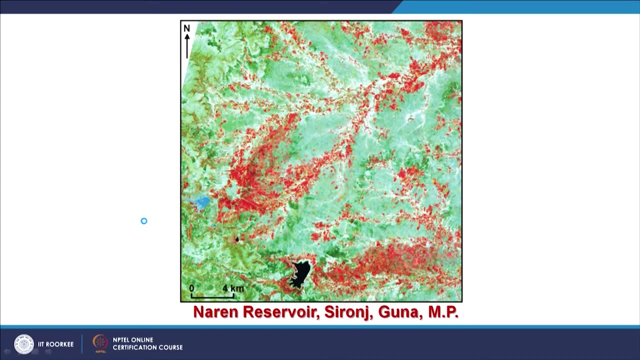 one is the Sironj River. There is another. small-2 reservoirs are also here And this is hard rock terrain of central India Bundelkhand region. In the basement you are having nice Bundelkhand rocks, or granite if you wish to call, And on the margins you are having 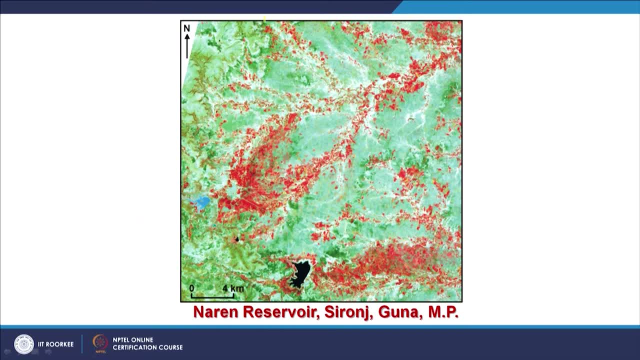 decontraps or basaltic rocks, Like here, you are having basaltic rocks in this part And in this part you are having weathered basalt and of course you are having thin soil and that thing. But the point which I wanted to, or the things which I wanted to show you, that see these, 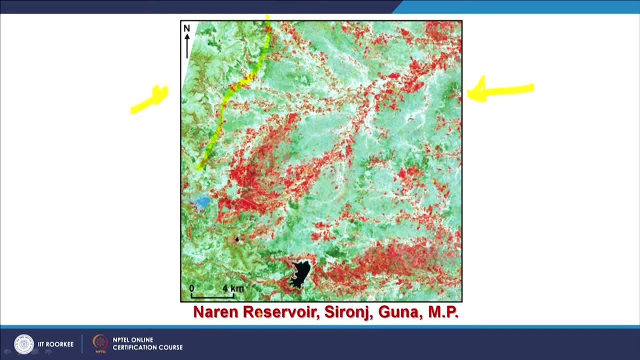 reservoirs. This is a Indian remote sensing satellite image, IRS list 3 image, and it is a false colour composite And therefore the vegetation is appearing as in red colour because infrared channel, which is having the maximum reflection, has been assigned red colour. So what you would see that 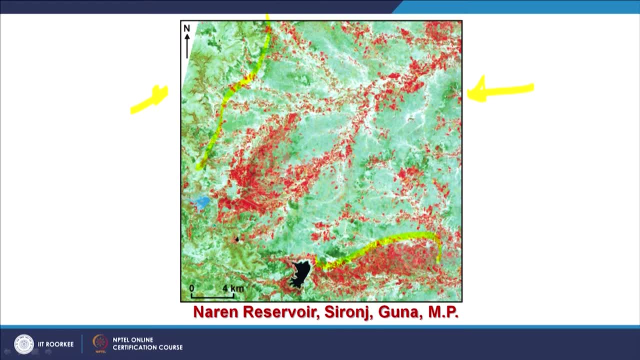 there is a reservoir and in downstream I am having an area, influencing area, or I call the benefit area. There is a reservoir, This blue colour one, and then I am having a benefit area like this, But the interesting part, the reservoir which is having larger 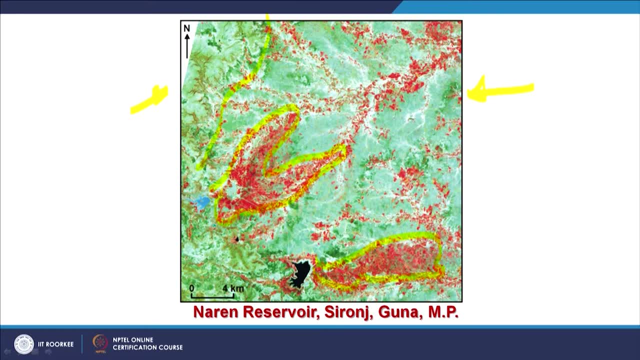 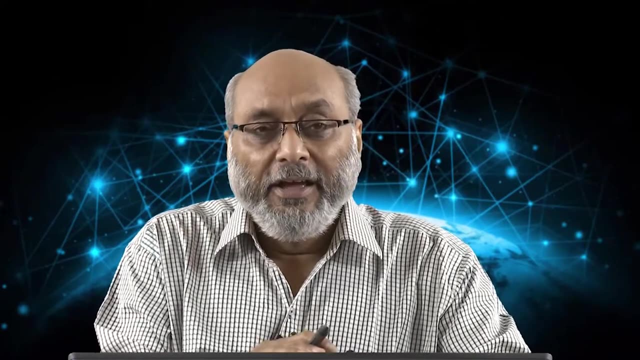 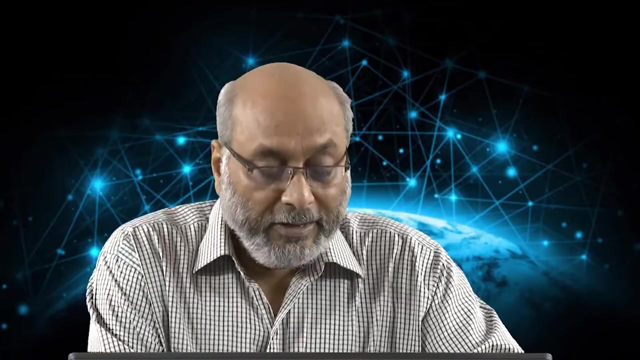 inundated area having less benefit area as compared to the reservoir which is having the small inundated area. So what could be the reason? Because by analyzing satellite images, interpreting satellite images, we are developing a knowledge about local groundwater regime. Local knowledge Since in these areas you do not have any reservoirs and therefore 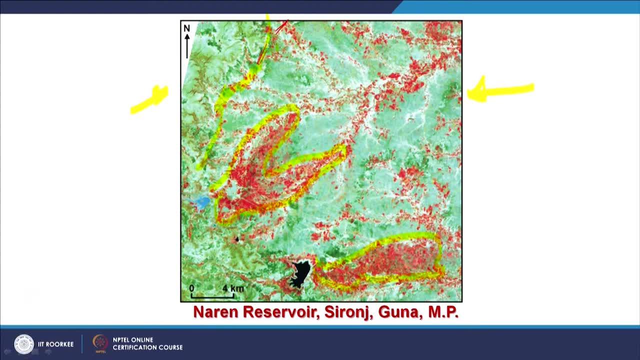 there is not such growth of vegetation as we are seeing in the other parts. So in future, if we want that these areas should also become green or, in false colour, composite red, then what do you need? You need similar kind of reservoirs along this area as well across these. 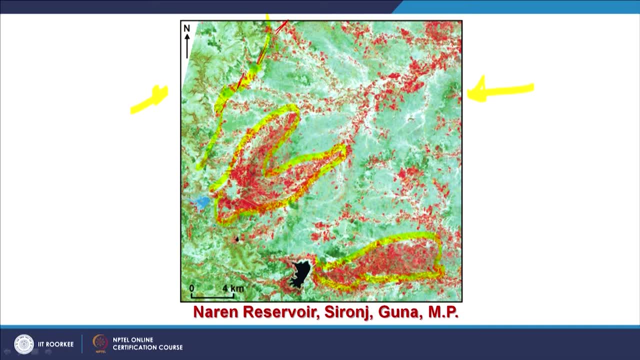 valleys or alluvial fields. These are all ephemeral channels and which have been blocked. the rainwater has been topped and then you are getting groundwater regime because there is no lift irrigation, there is no canal irrigation or any other thing, simple reservoirs. 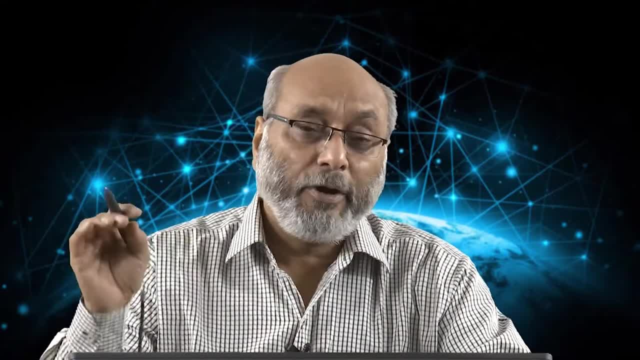 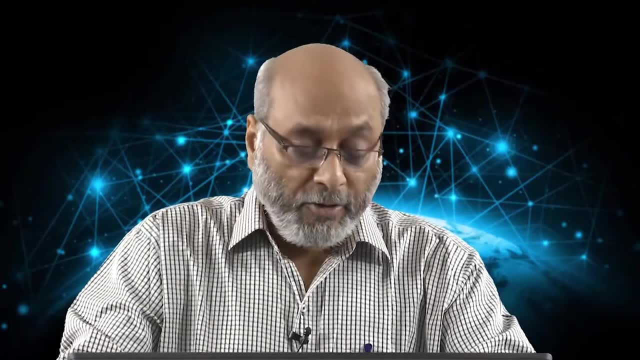 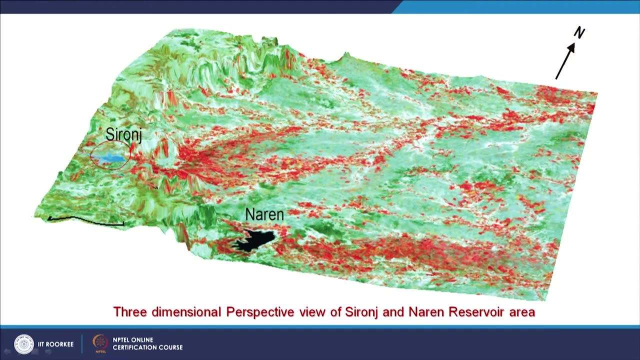 And they are recharging groundwater regimes. Farmers are exploiting that water and putting in their fields to get the crops. This is February-May 2. Now, if you see that this blue coloured reservoir, though in size, in small, but it is located in relatively on higher grounds as compared to this Narayan reservoir And because of 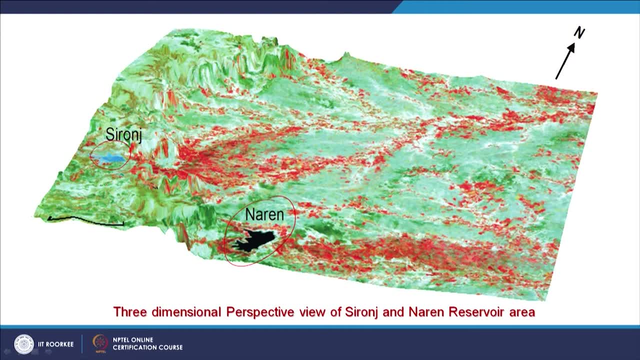 there is an elevation difference that means this reservoir is providing better hydraulic gradient as compared to Narayan, which is almost in the same level. So if we want to make this area more green, then what we need to do- We have to learn from Chironge Riverway location and construct reservoirs on little higher grounds, Though. 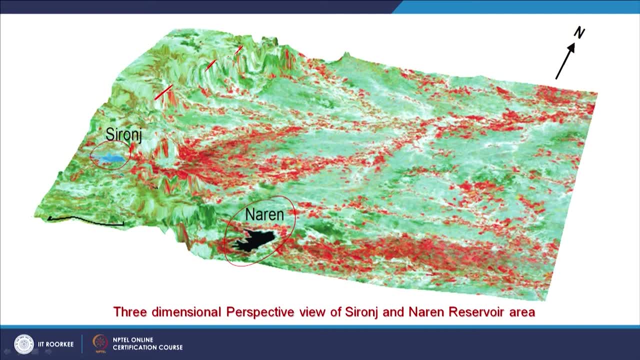 we will lose little. you know, we will have a less size of catchment watershed for these reservoirs, but nonetheless they will provide better hydraulic gradient and better groundwater recharge. Otherwise, geology wise, all these reservoirs are green. The entire area is same, that on this side you are having decontraps and on this side 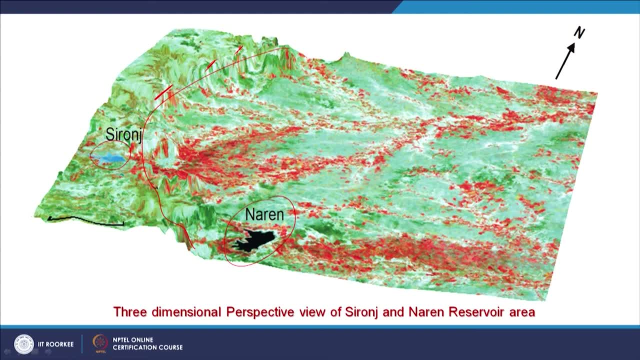 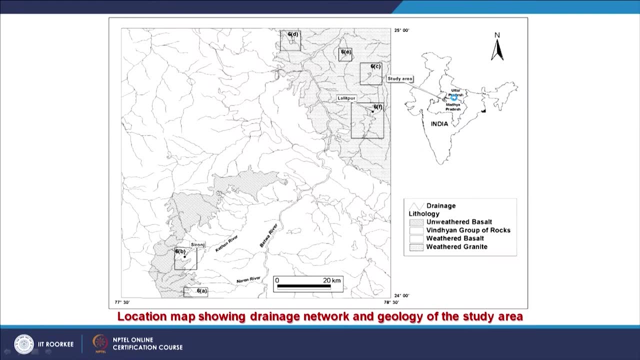 you are having granite. Of course there are some soils and developed and along which agriculture is taking place, So there are many such reservoirs in this area. So if I cover a larger area, those Chironge and this other reservoirs are still here, which you can see: Narayan Reservoir. 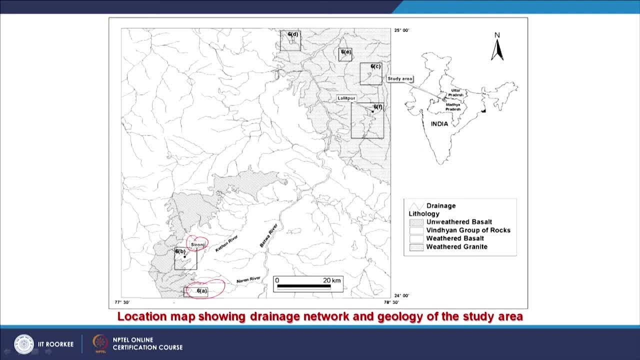 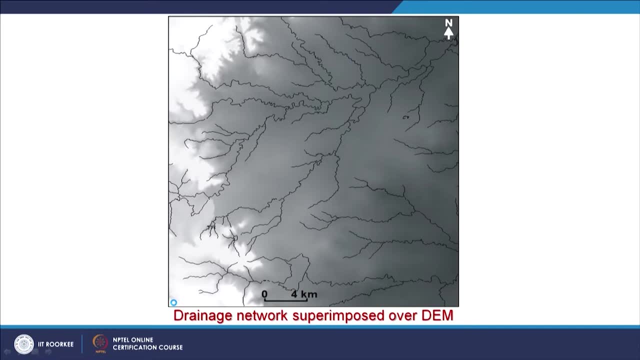 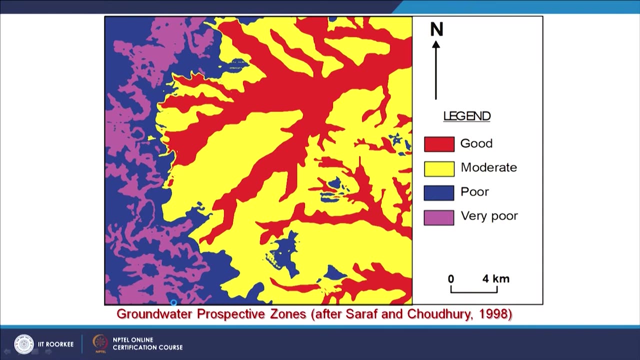 Narayan Reservoir And Chironge Reservoir, But I am covering now a large area because it will carry some important things. If I see a digital elevation model, it looks like this for that area, So implying GIS and giving weightage to different themes or different layers, like, for example: 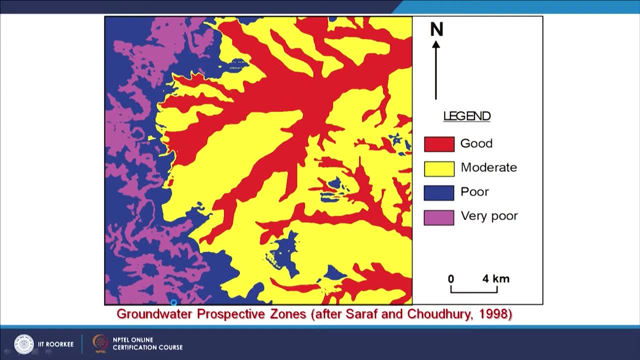 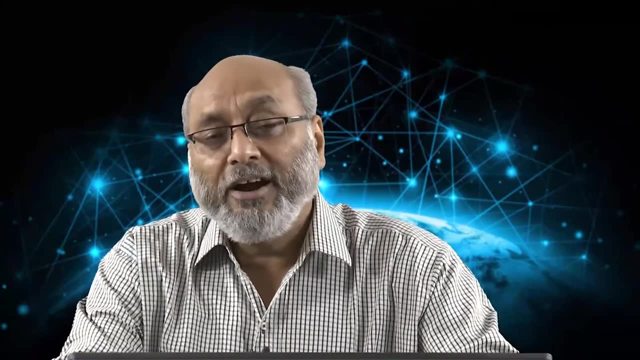 geology, soil geomorphology, water level or changes in water table between pre-massage monsoon and post-monsoon, and using this groundwater yield of different rocks, a similar kind of maps for any hard rock terrain can be prepared, which are groundwater prospective zones. 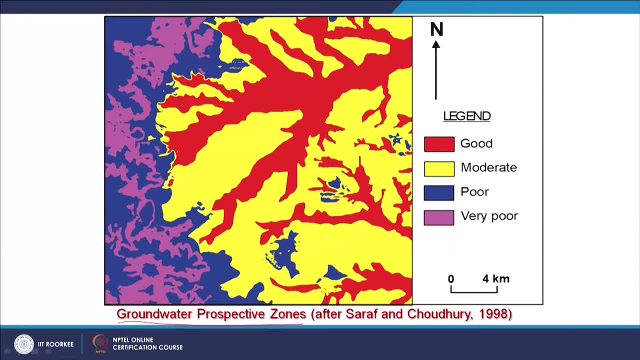 That means if anybody is looking for a well or siting a well, then these red areas are the best suitable And whereas if you go in the high, in the decontrap area, these are the areas. These are not suitable at all. So very poor and poor colour are those areas which I was. 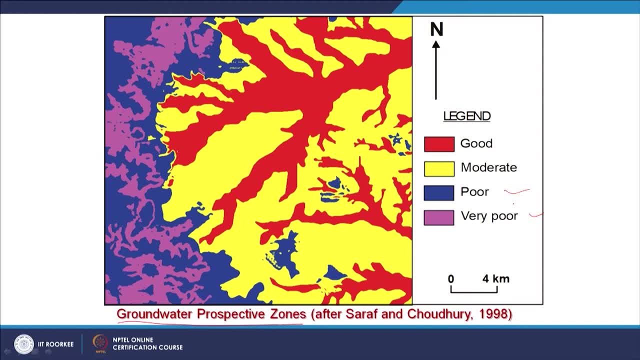 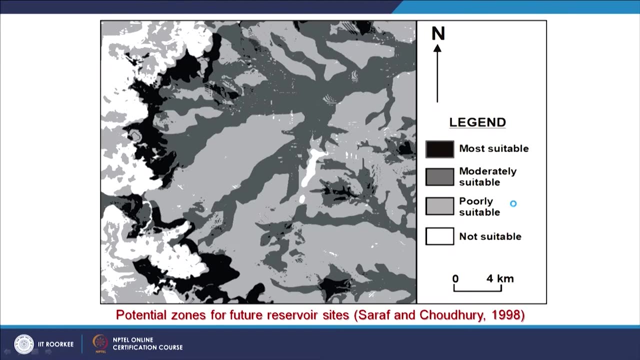 saying about the basaltic rocks. Rest of the areas are either moderate or good chances of getting water. So these alluvial fields along these ephemeral channels are good to get the water. There are high chances. Similarly, using again and little different techniques, 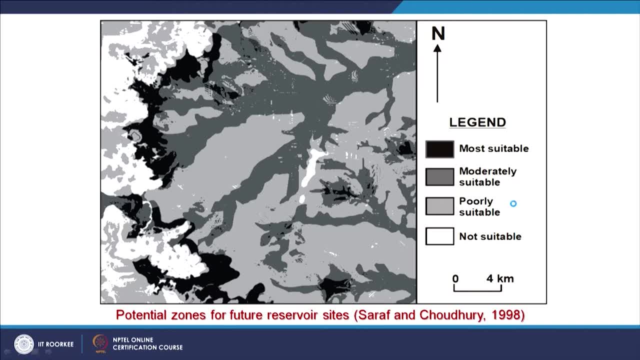 with different weightages. we can also develop maps for any area in the country which is the potential zones for future reservoir sites, in order to recharge the groundwater regime Again. the dam simulation will come here directly. So these are the areas. the black one are: 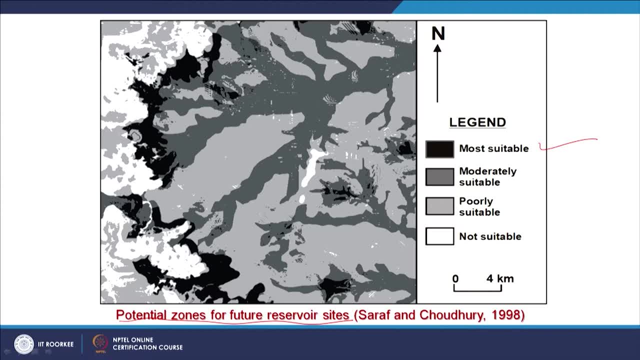 the one which are the most suitable, Not at the same level, but little higher and not too much higher. Therefore, the water level is very high. So these are the areas which are the most suitable, Not at the same level, but little higher and not too much higher. that 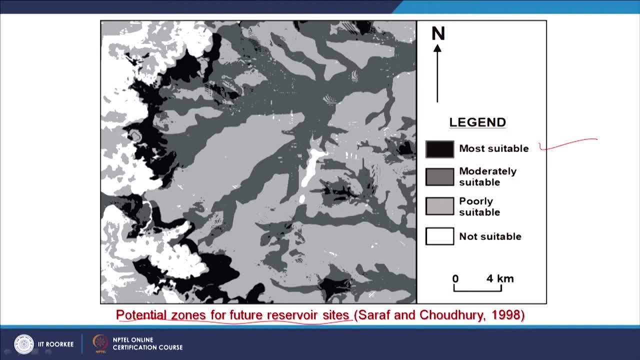 is why the water set becomes small, So just at the edge of those higher grounds. because we have learnt through that Blue Reservoir or Chironge Reservoir that if it is located on high ground it will have large benefit area relative to submerged area. So that knowledge we developed and based on that knowledge, 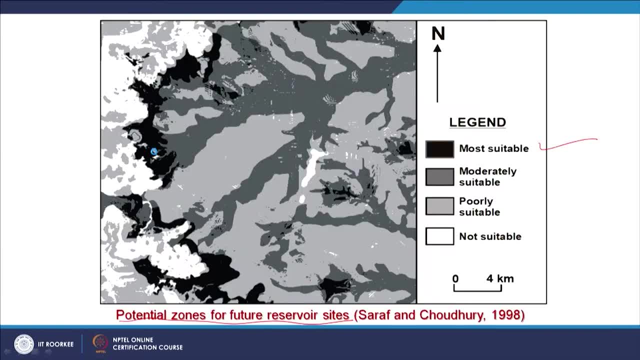 we can develop such maps. These are nothing but the modelling. GIS based maps are the most suitable, So that knowledge modelling, getting information, arranging the information, putting in different layers, giving the weightage and finally coming with 2.. So 2 outputs I have shown. One is: 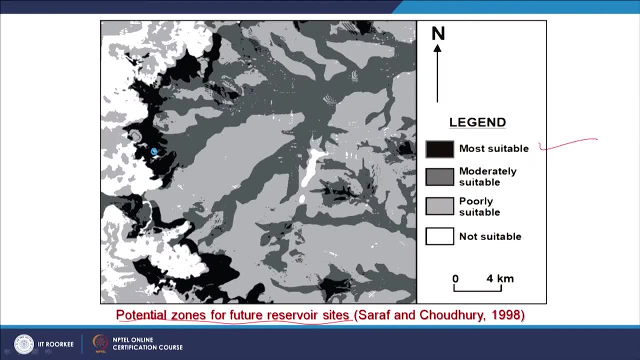 the prospective zone, groundwater prospective zones- and another one is the groundwater recharge structures, locations where you should locate. Now the weightage which we have assigned to different layers or different categories within one layer can be different in different areas, So each area has to be studied first through. 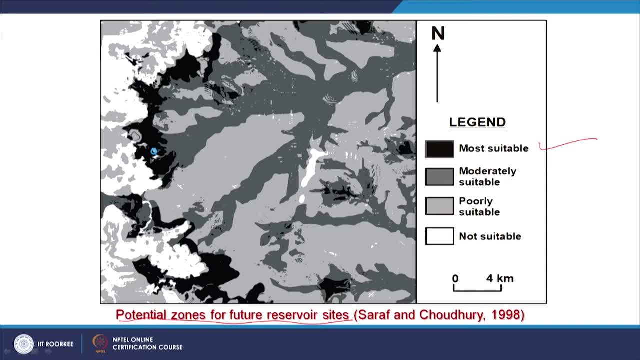 satellite images, getting some other datasets, preparing such thing, and then you can do it. The biggest advantage you can take of already existing reservoirs and studying them, that what is the submerged area, what is the benefit area, and then you design your weightage. So it is a very easy task. So you can do that, So you can design your weightage and you can design your water levels. Okay, So this is a very easy task. So this is a very easy task. So this is a very easy task. 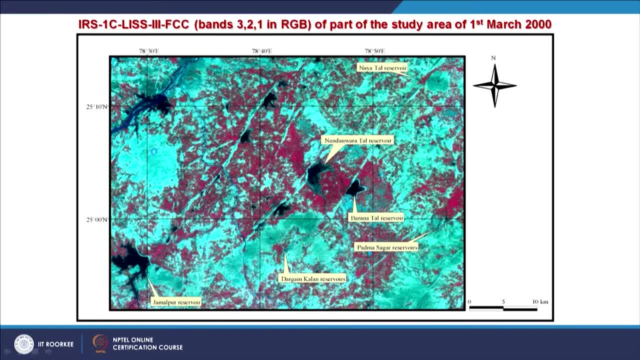 baits for different themes. Now we are still in the same area and exploiting something else. Here you can see lot of small-2 reservoirs are there just to locate. this is the Bethwa river, which is going something like this And we will meet the Chambal and then Chambal. 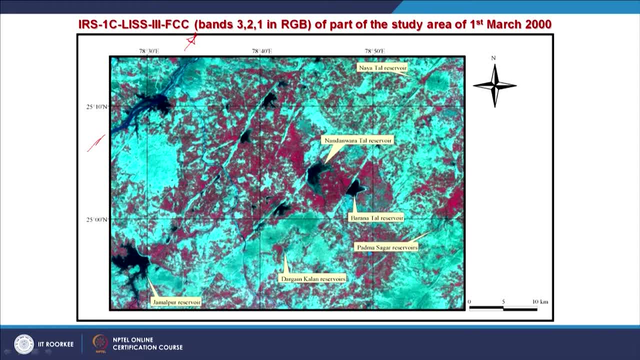 meets Yamuna, Yamuna meets Ganges. Now, these white lines which you are observing here, these are the quartz reefs. These are geological structures which are already present and which are serving as a dam access, very long dam access. So people in past have exploited. 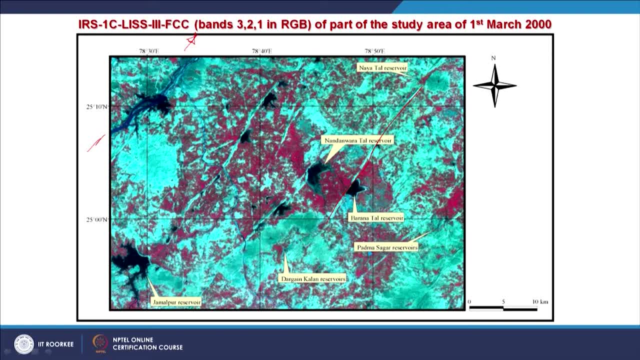 these quartz reefs and could create small-2 reservoirs, Some might be even natural one. And wherever you do not have such quartz reefs and inundation of water, like in this part here, you do not see vegetation. This is again false, clear compositing. So what we are learning. 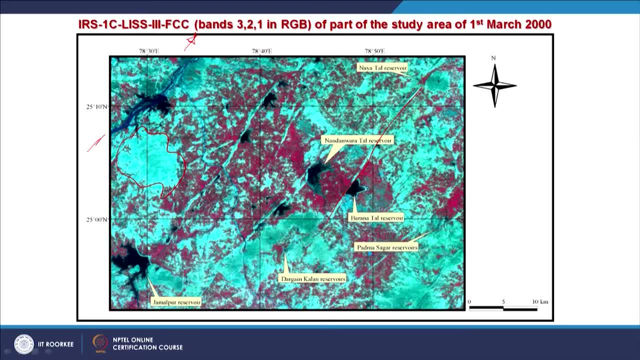 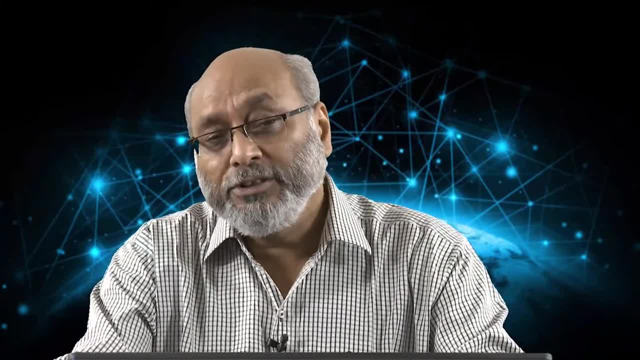 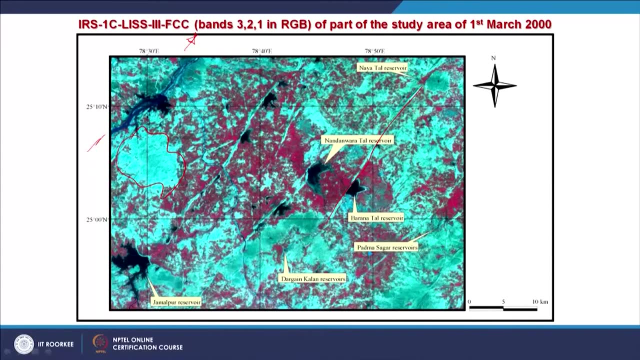 basically that if there is, even in a hard rock terrain, if we inundate water for some time, it will recharge groundwater regime in the surrounding, whatever the geological conditions are there, And ultimately there will be growth of vegetation, as you are seeing also in this image. So wherever you are having water in that vicinity of water you are having, 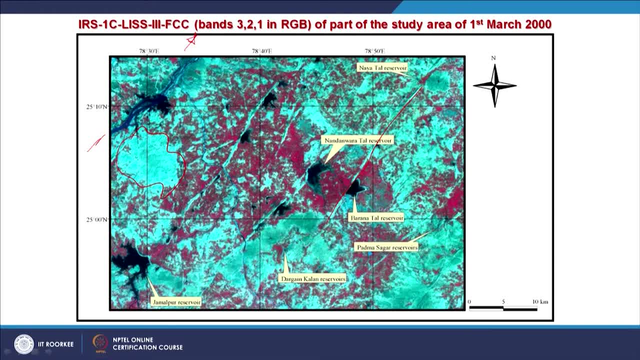 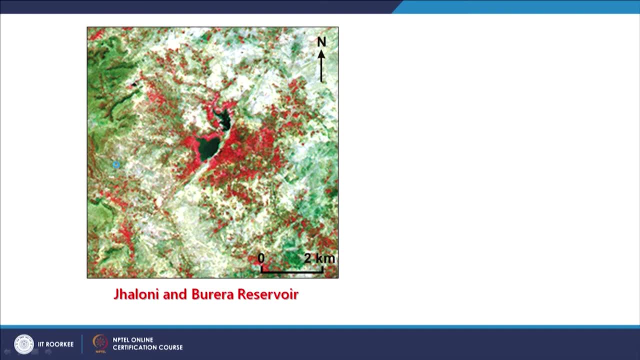 growth of vegetation and wherever you do not have any water body, you do not have growth of vegetation. If I take Nuzul reservoir, you can see that. see, this is the quartz reef, which is going something like this north-southwest direction and this is the downslope side Along the reservoir. 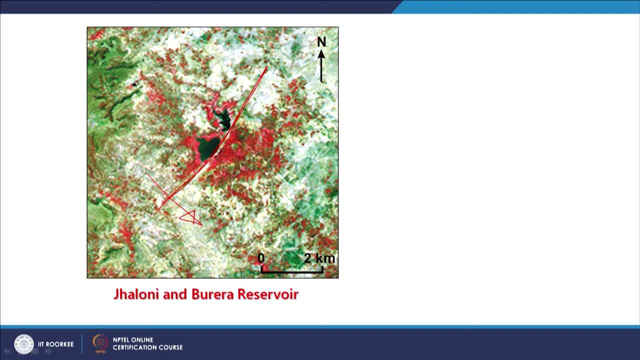 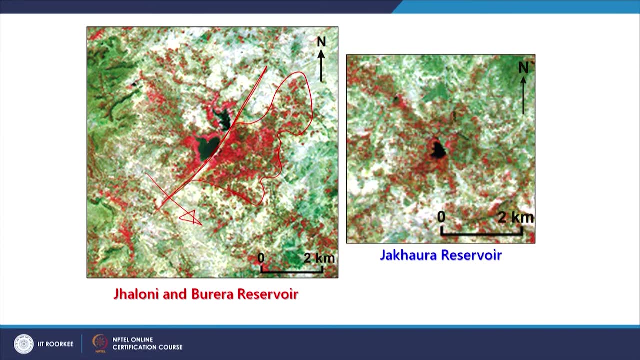 in the upstream area, especially in the perimeter of the reservoir, and in the downstream area you are having a benefit: area 12.. Likewise, another example, and here what you are seeing in 4 directions: the water is available in form of groundwater and farmers are exploiting to put on their fields. 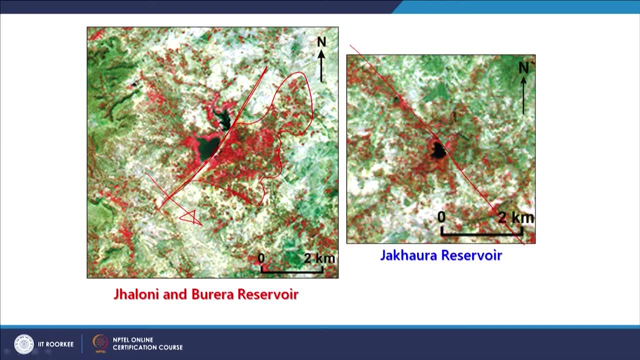 And that one is in the northwest-southeast, another one is northeast-southwest, Because these are the geological structures which are controlling this. northeast-southwest is generally the trend of these quartz reefs And whereas northwest-southeast are the geological dikes which are present there. 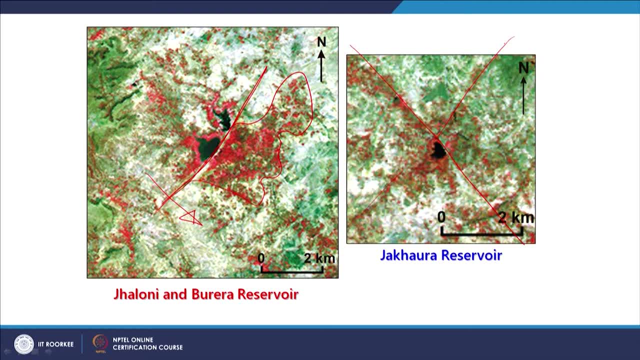 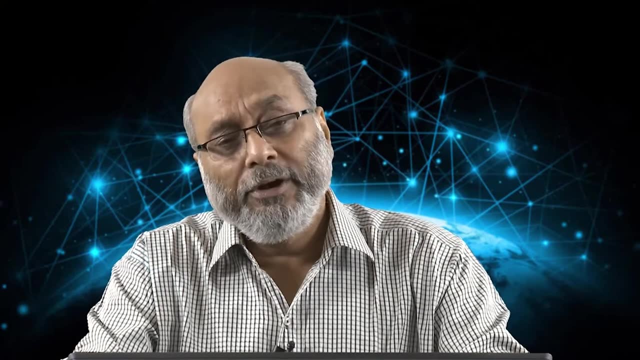 So only along there is a maximum movement of water. otherwise in other part there is no harm, because- remember the early discussion, what I mentioned, that there is a quite sufficient rain precipitation over India. The only thing we should hold: delay the runoff as much as possible. 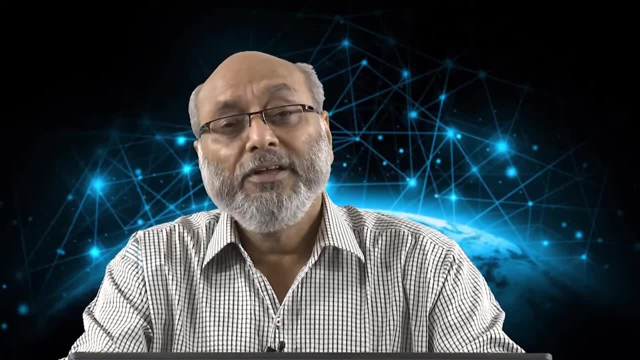 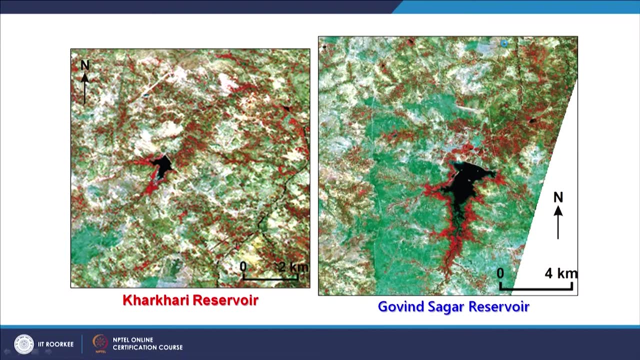 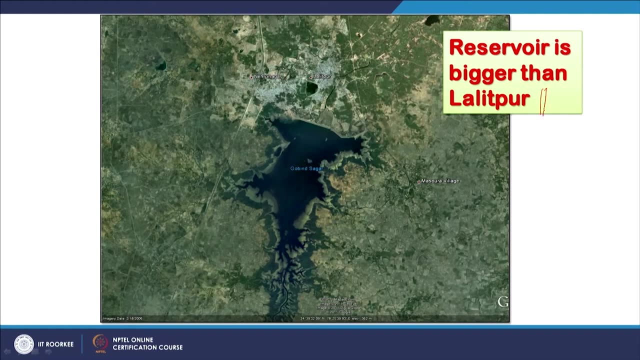 If we do it by few months, it will recharge the groundwater Few. more examples are here. One more example is here, and here I would like to spend some time, because this is my hometown in Uttar Pradesh And this reservoir was constructed more than 60 years back. 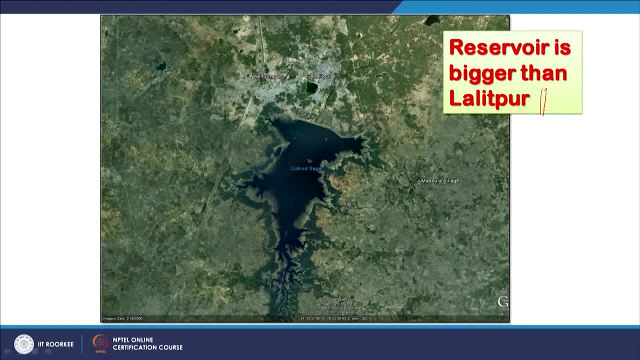 And at that time the population of this town was roughly 35,000. And so there was a lot of rain, And so we have to wait. Since then, because of siltation and encroachment, the size of the reservoir has reduced. 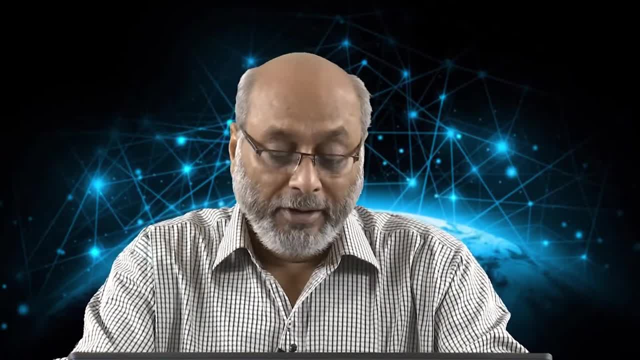 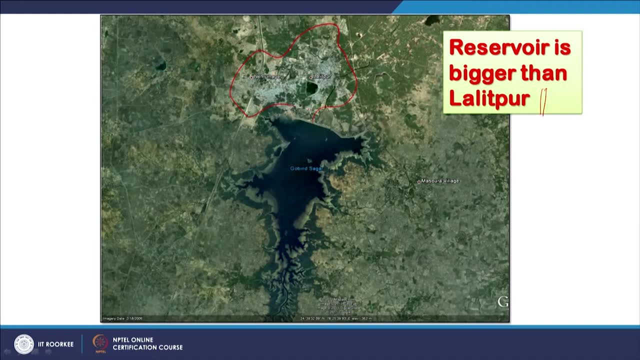 That means the capacity of holding water has also reduced. But the population in the downstream of reservoir has increased by manifold. So earlier we used to get 24 hours water in our taps. Now we do not get even for 24 minutes. But recall again: the input which is coming in form of precipitation over India remains. 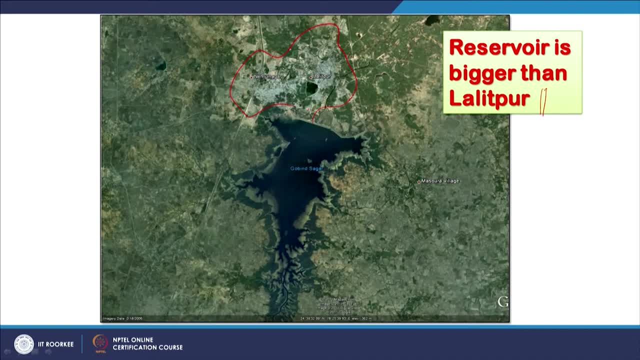 same, Only our management has got poor. We did not augment in the same way as we added to the population. Nothing lost. Still, if we start doing this thing in 2-3 years time, we can solve this problem. How we can do it. 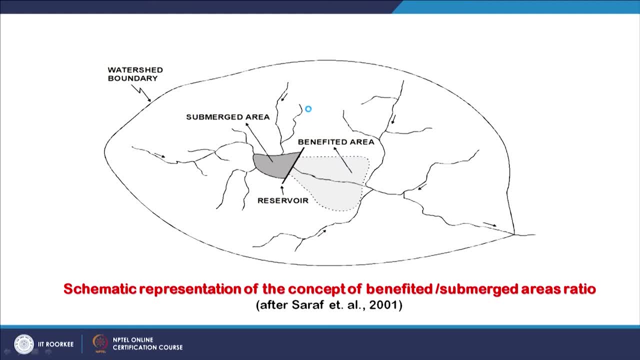 We can quantify things also because many decision makers they love the quantities rather than qualitatively. So that can also be introduced by taking a ratio that is benefit versus submerge ratio, And this index can be used. So what we did, 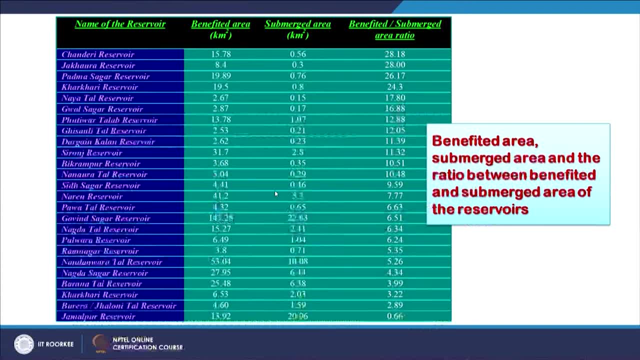 We took 21 reservoirs of that Budhil Khand area and calculated this benefit versus submerge ratio, which is on the rightmost column, And as you can see that sometimes you are getting 28.18.. So that is the number. 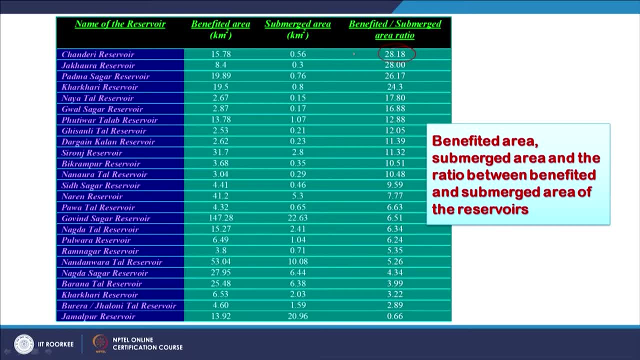 That means, if I sum in this particular area where currently this reservoir is there, the Chanderi one, If I submerge 1 square kilometer of area in the vicinity of this reservoir, there are chances that I will get 28 times return in form of benefit area. 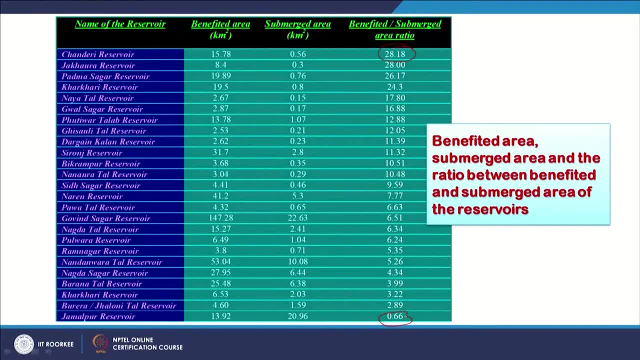 It is a wonderful scheme. However, there are locations where this ratio is less than 1.60.. So there are locations where this ratio is less than 1.60.. So there are locations where this ratio is less than 1.60.. 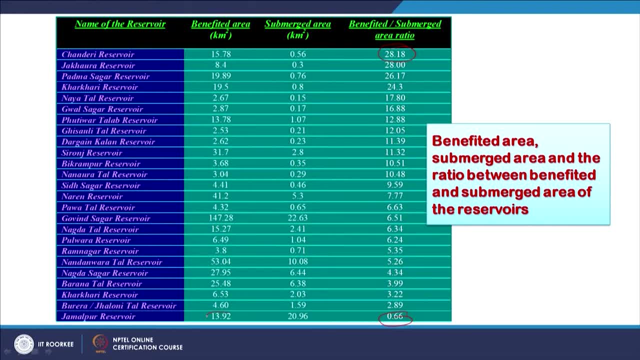 So there are locations where this ratio is less than 1.60.. That means these are the not areas which I should put my investment of land. But if we decide that my threshold is, say, 10, I need at least 10% return in form of. 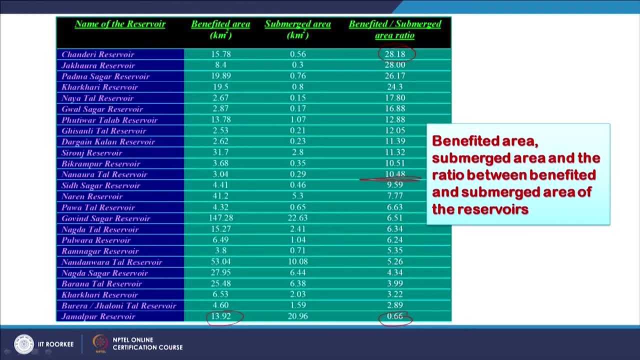 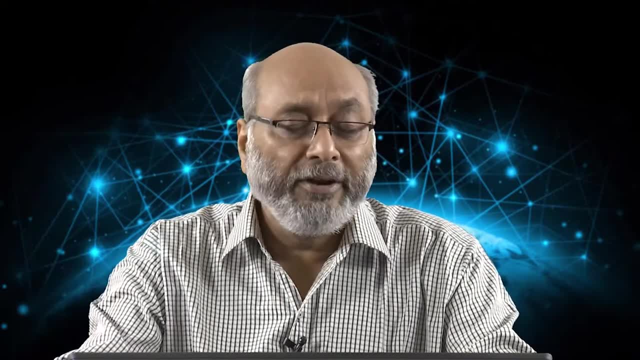 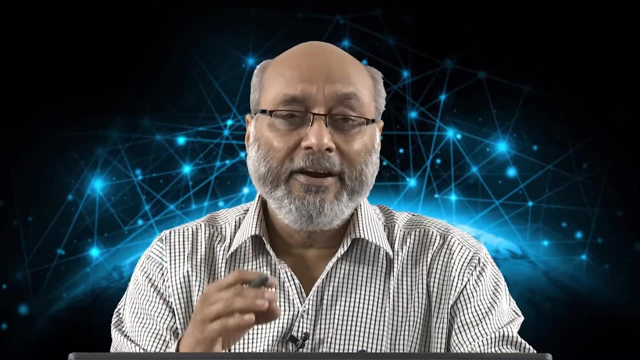 benefit area. That means again I will repeat- that if I submerge 1 square kilometer of land, I should get in return at least 10 square kilometer of benefit area. That means about more than half of the area. That means about more than half of the area can give us return in terms of groundwater. 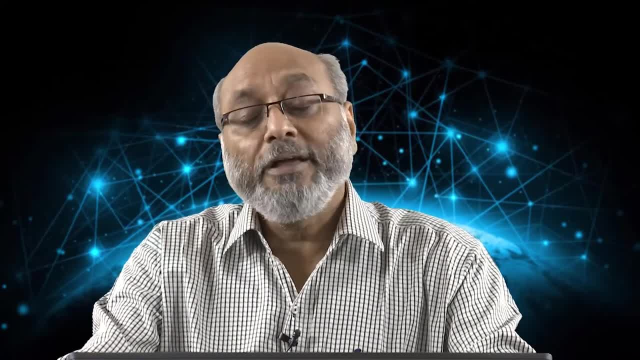 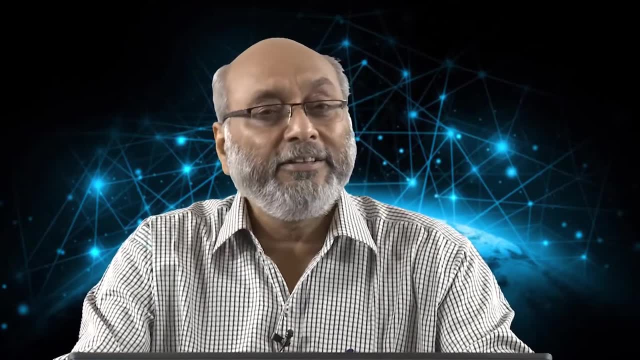 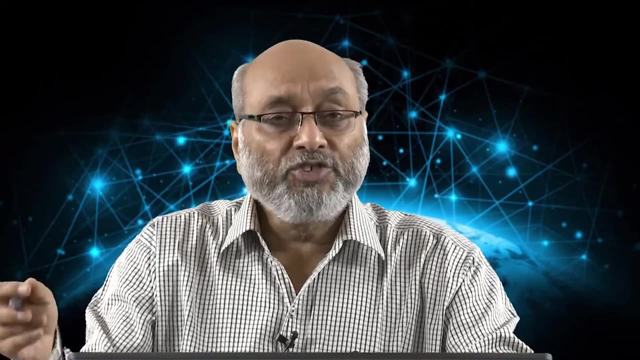 recharge by 10 times. in terms of land, Important thing is that reservoirs or dam access has already been created by the nature in the form of quartz reefs, So we have to identify only those areas where a stream is breaching these quartz reefs and 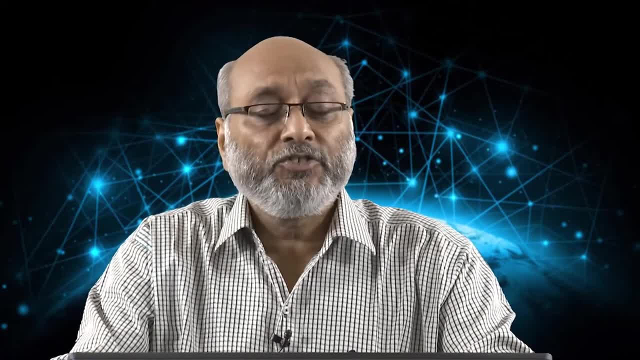 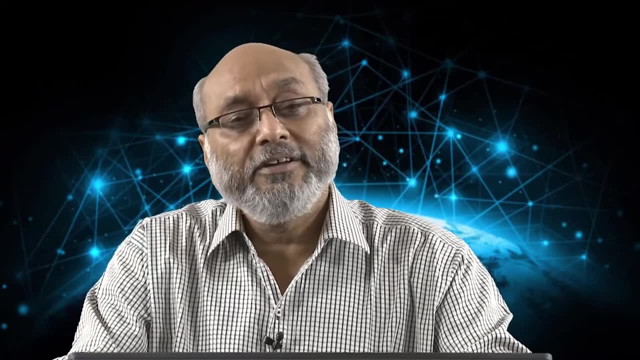 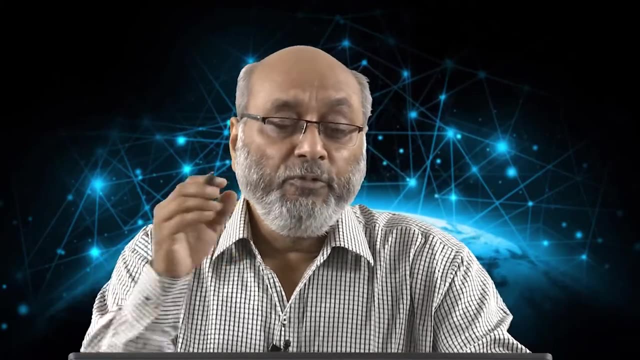 still unchecked. So if we block that stream, create a earthen dam, small earthen dam, We will delay the runoff, we will start recharging groundwater regime And, as I have been saying that, if we start doing this thing today, in 2 years time, in. 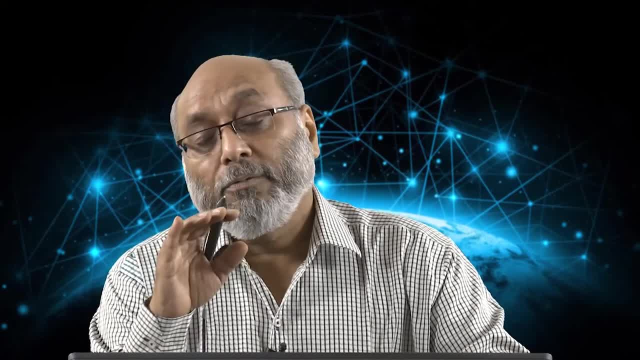 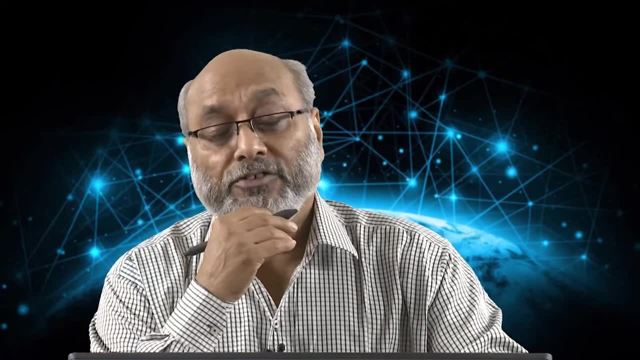 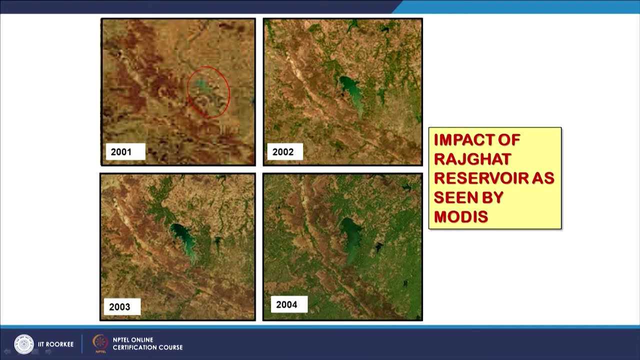 that particular area. this problem can be solved to large extent, And, as you know, that satellite images provides unbiased recordings of the things, But in this example, what we are seeing, though, is a larger reservoir, which is also called Rani Lakshmi Bai Reservoir. locally, it is known as Raj Ghat. 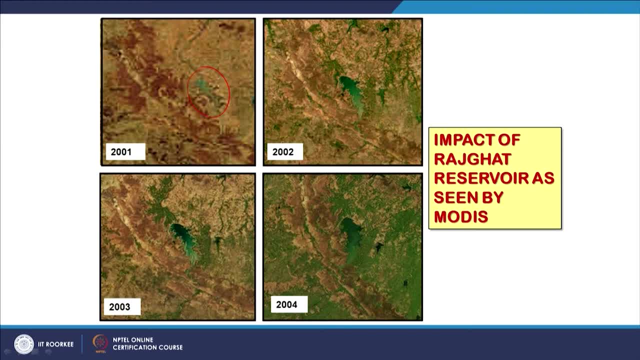 So this was started just fling in 2001,. the entire project was not completed at that time. Next year, that in 2002, started to its maximum height. If you notice that these are the true colour images from a MODIS sensor, 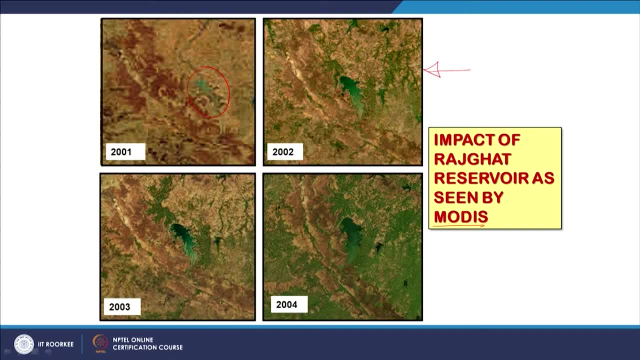 And what you would see? that in 2001,. hardly there was a growth of vegetation Here. you have started seeing greenery in 2002, remember, just in one year. If you go in the third year or 3 years after that, you would realize that the entire area 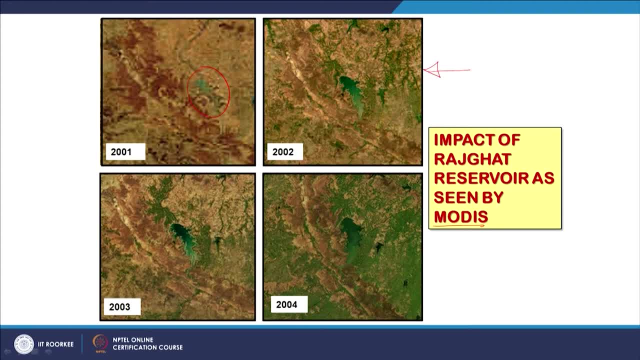 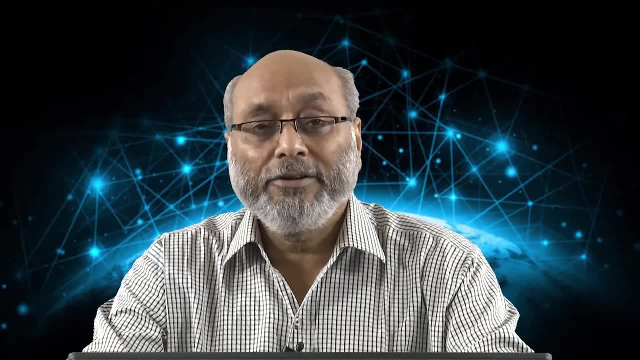 has almost become green. So compare this 2001 with 2004,. you will get the answer that how many years it would take To recharge groundwater regime in a hard rock terrain like Bundelkhand area? just 2 years. 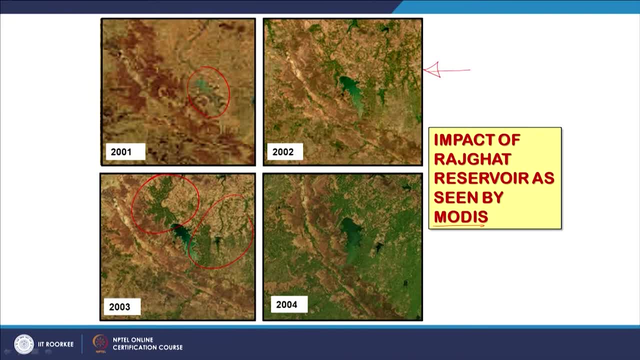 After 2 years, as you can see, a large area is getting benefit because of this reservoir. So when I was showing this to in some meeting, this particular image or set of images, series of these time series images, people said that for 2001, you might have taken a pretty good. 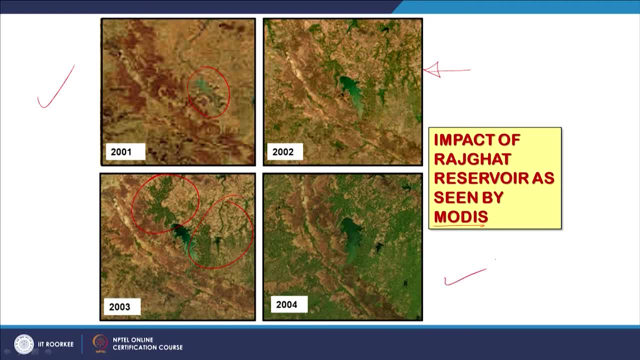 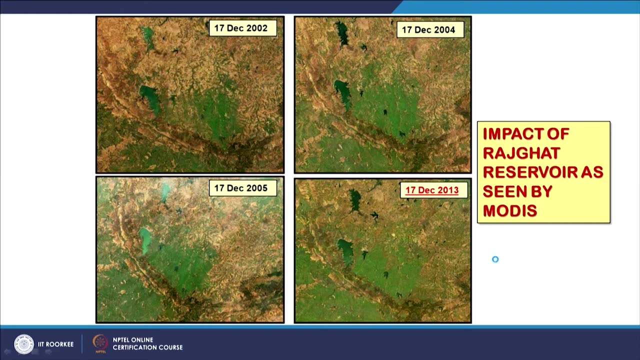 pre-monsoon image And for 2004,. you have taken a post-monsoon image and then you are showing the differences. I said: do not worry, As I have said, the satellite images records unbiasedly. So this is all 17 December of different years. 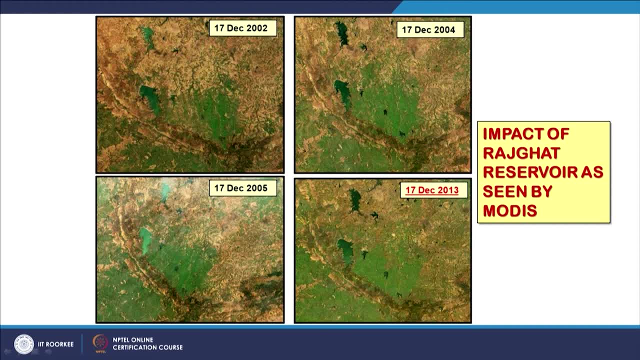 And, as you can realize that this was just one year after the reservoir filling. you see the greenery here and in this part also, And slowly-2. 3.. So in 2013,- this is the area- has become green. 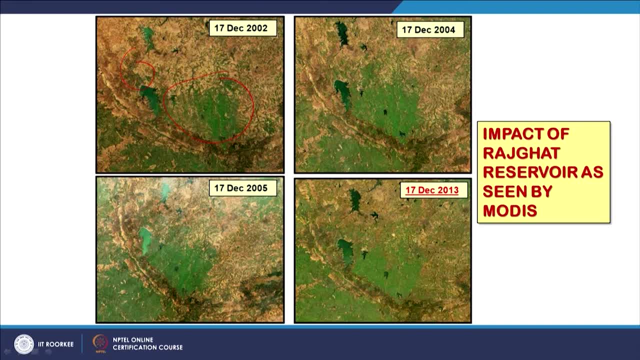 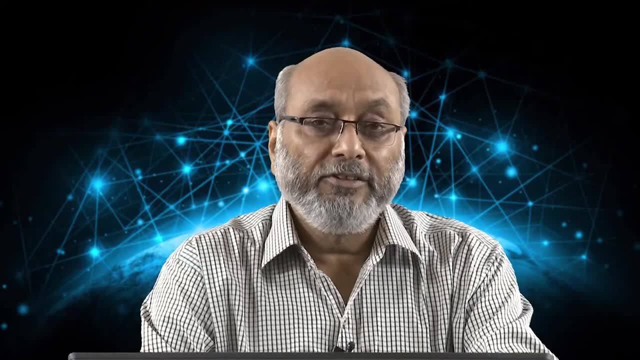 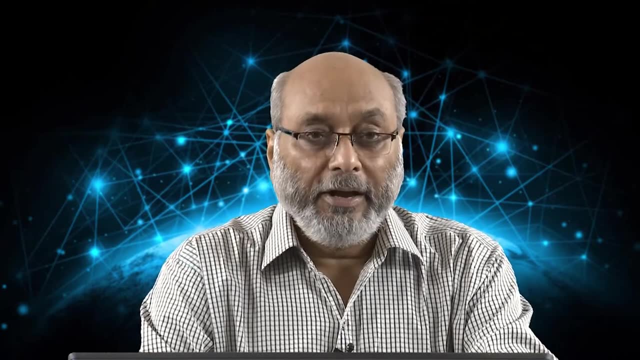 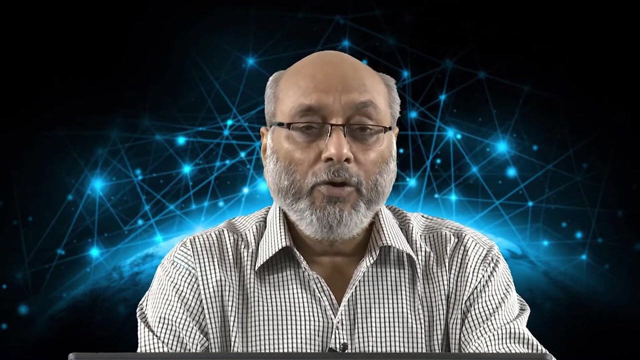 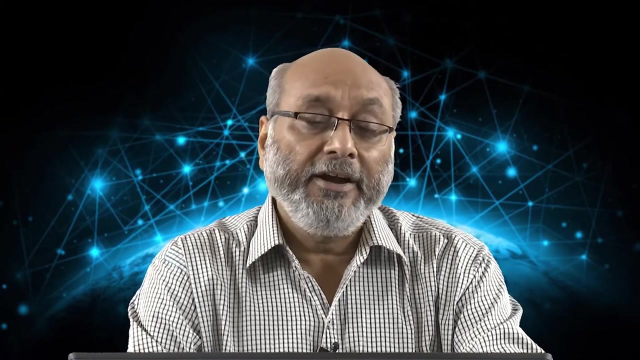 There is another evidence of this: that these Mandis, or local, where the farmers bring their grains for selling a wholesale market. When this reservoir became in existence and started recharging groundwater regime in the next year, The local Mandis or these wholesale grain markets could not handle that kind of output. 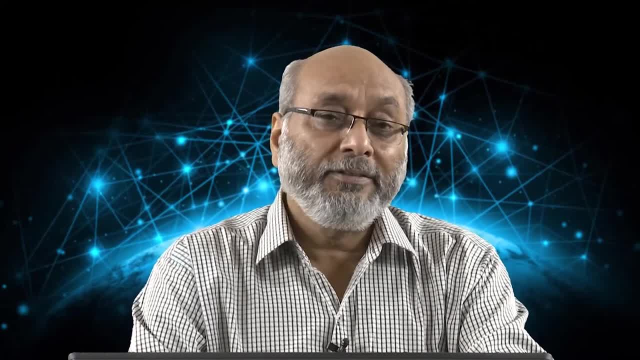 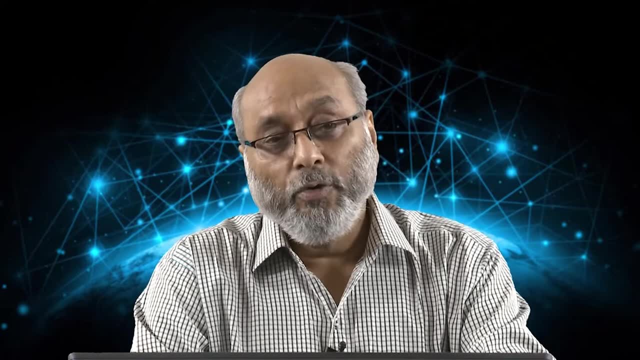 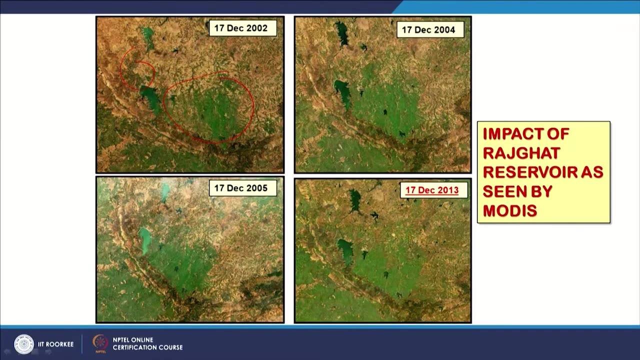 because the land was there, soil was there. The only problem was water. As soon as water started coming to the farmers in their wells or through canals, the crop after crops started coming. That means just if we recharge groundwater regime, Even for few months, few weeks, it will have effects in downstream or in the vicinity. 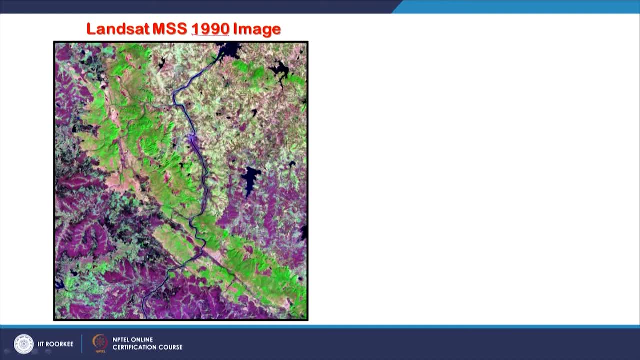 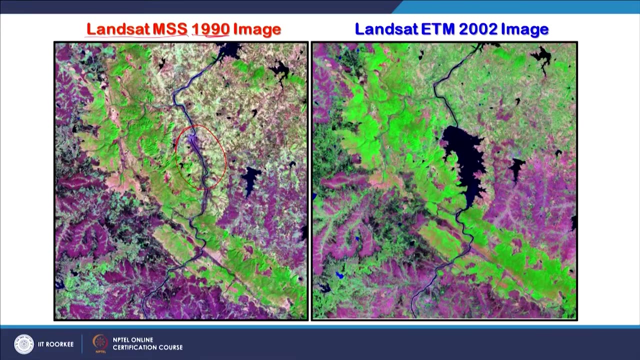 One more example from the same reservoir. This was the year 1990, from Landsat-MSS images. This reservoir was just. this project was taking shape. and see what happens. This is 2002.. A large area became green. This is again true colour images. So a reservoir, does not matter, even if it is small or large, will recharge the groundwater regime, particularly in hard rock terrain, And the benefits in the downstream or in the vicinity will start coming in 2 or 3 years time. And this is the joy of water in the area where these people did not have water and sufficient. 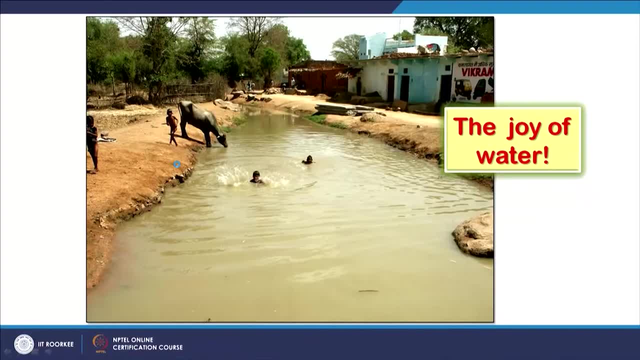 rain was there. And see, these are unlined canals And because of unlining of these canals, whenever there is a water, they too recharge the groundwater regime. So even if for one month there is a water in these canals, these canals will recharge. 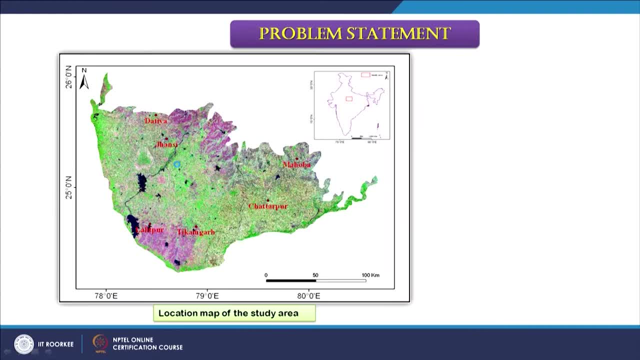 the groundwater regime and your groundwater is getting enriched. So we can solve this problem for a large central part of India Just exploiting these canals. So we can solve this problem for a large central part of India Just exploiting these canals. 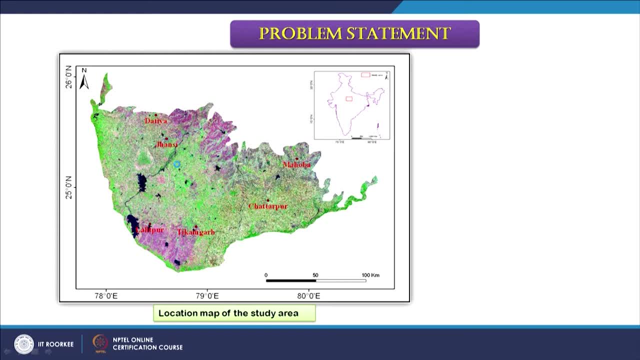 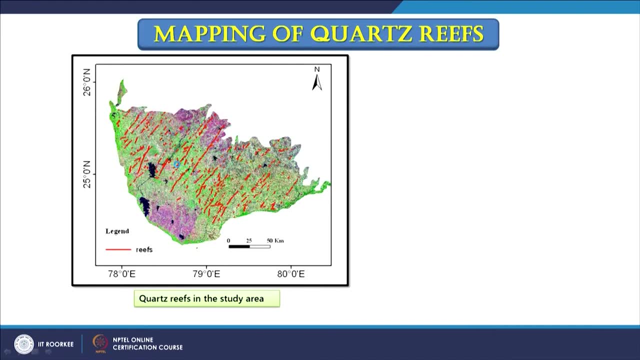 So we can solve this problem for a large central part of India Just exploiting these canals. Just exploiting these canals. See, we are studying these quartz reefs which are running North-East, South-West in a large area was studied And we delineated these quartz reefs like this red, which are marked here. 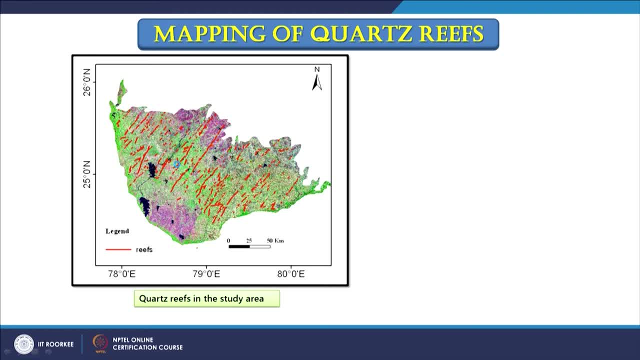 There are. some of them are running for hundreds of kilometers. See the scale here: 50 kilometers. So like this one, roughly it is running for 80-90 kilometers. See the scale here: 50 kilometers. So like this one, roughly it is running for 80-90 kilometers. 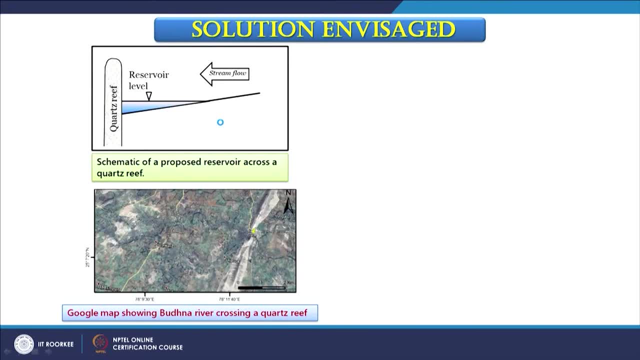 orientation of all these quarries. So basically, this is how in a zoom part in satellite images these looks: A stream is going unchecked. So if we block, using local materials, we can create a small reservoir- not multi-purpose, not for hydro power. 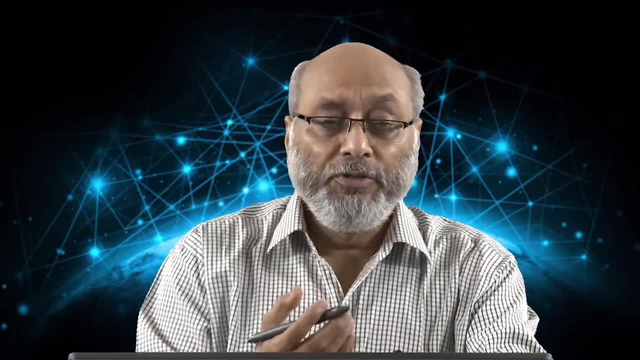 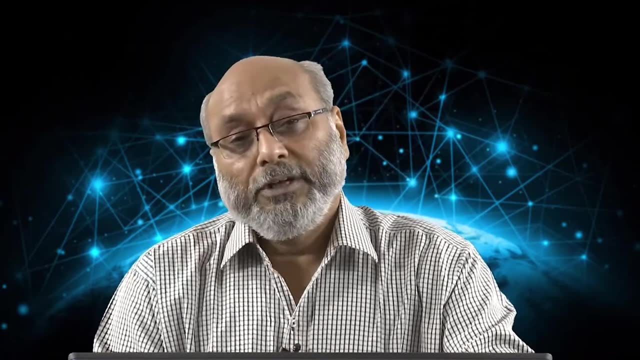 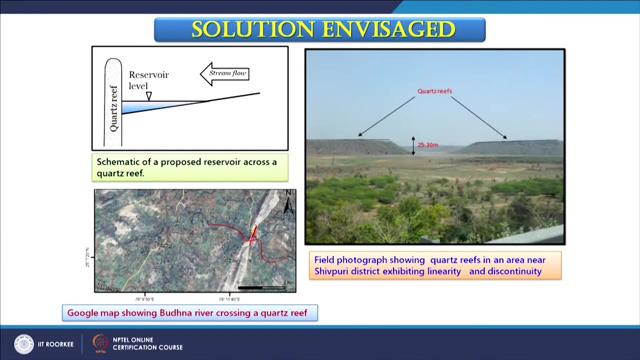 Only for the groundwater recharge, And the dam simulation which we started can be done here at this stage to convince people that this is what is going to happen. So if you go on the ground, this is how you see these quarries. This is all natural and the height here is 25 to 30 meter. 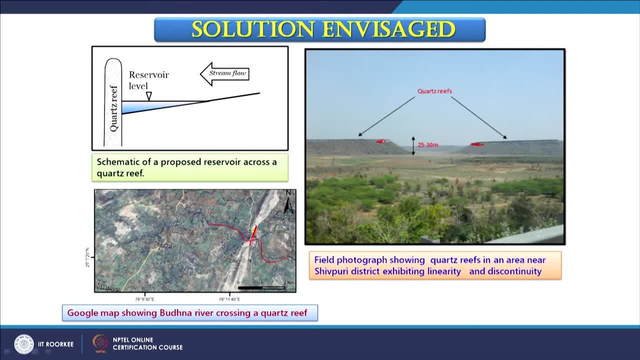 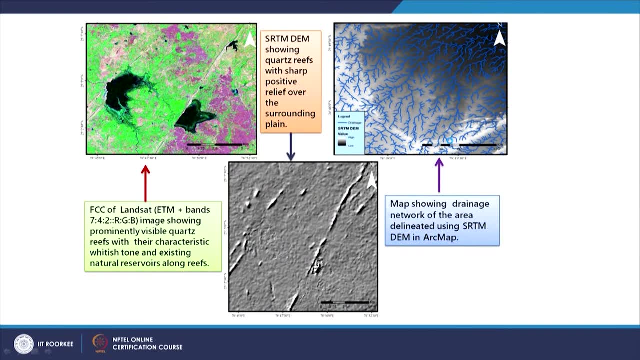 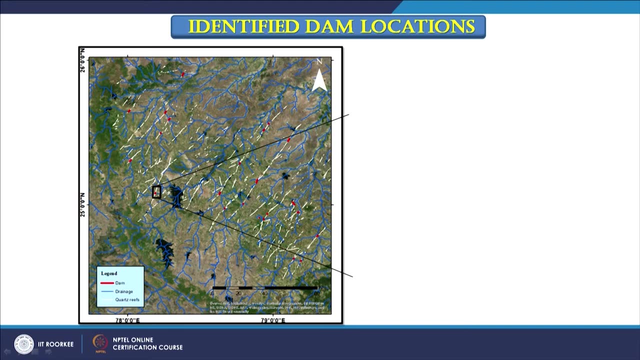 So these abutments can be used to create a reservoir. So this is what we simulated and then predicted that one That these are the areas in that locality, these red one which are marked here, are sites for potential reservoir sites and especially for groundwater recharge. 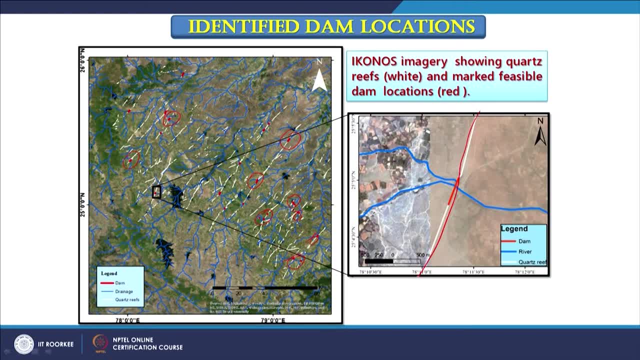 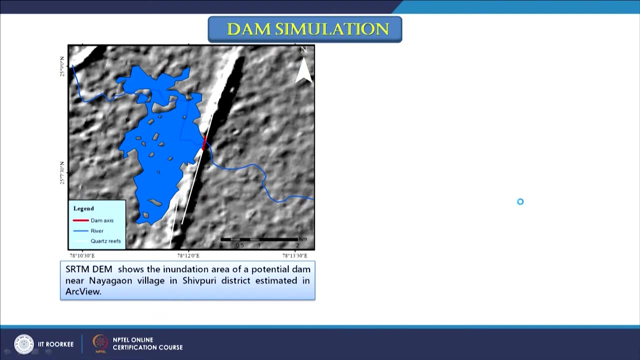 One is like this: the quarry reef is going like this. So if we block this one, a stream is going like this, coming like this, it will create a reservoir and we can simulate like this, which we have done In the background. it is shaded relief model for the same area And the blue. 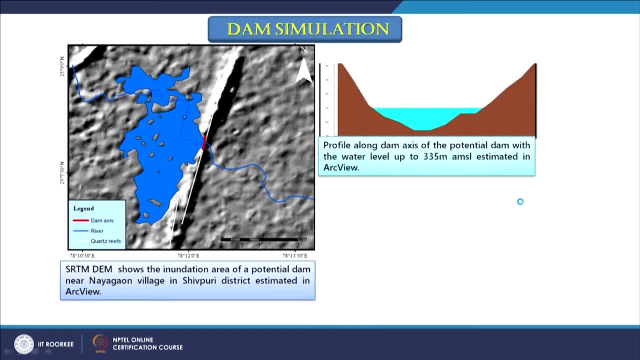 colour is showing the inundated area. Now there will be other things which we can achieve, implying further or do the analysis in GIS So we can change the height. Of course, if we want to exploit the quarries, then we cannot change the location, Only the height we can change. 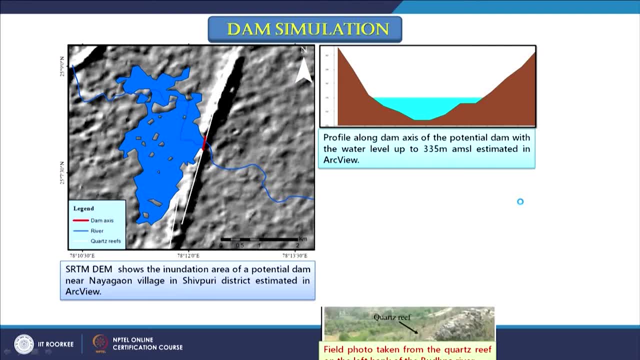 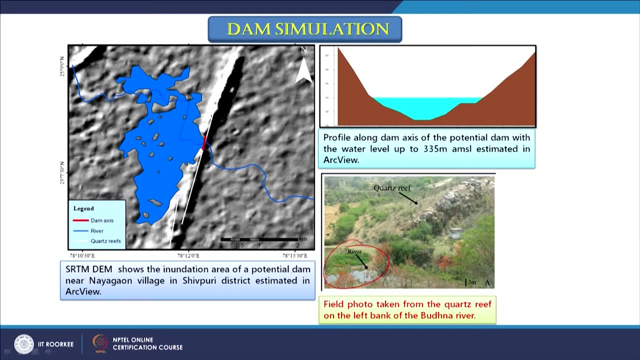 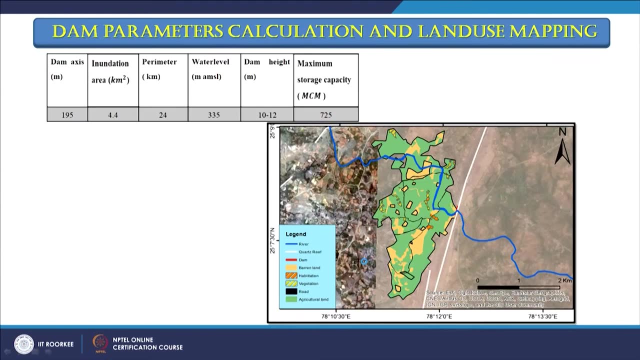 Does not matter, but still we would be able to inundate the area. This is how it looks more if we see closely in the ground. This is the water which you are seeing here river and this is how the quarry reefs are looking. Now you can also do a land use analysis: that which type of lands will get inundated if a 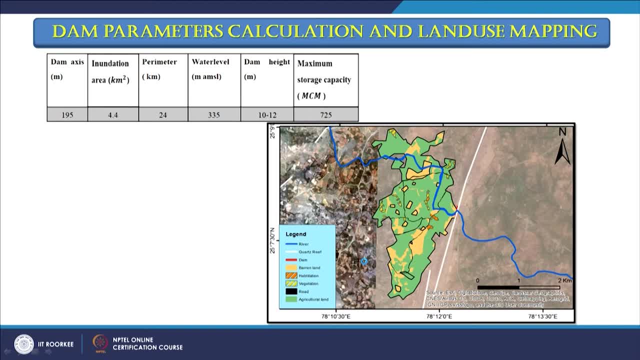 reservoir is constructed, All things are modelled, Everything is being simulated before an appropriate decision is taken. So immediately, implying the satellite images, current land use can be assessed. Land cover, land use can also be assessed, as has been done for this case. 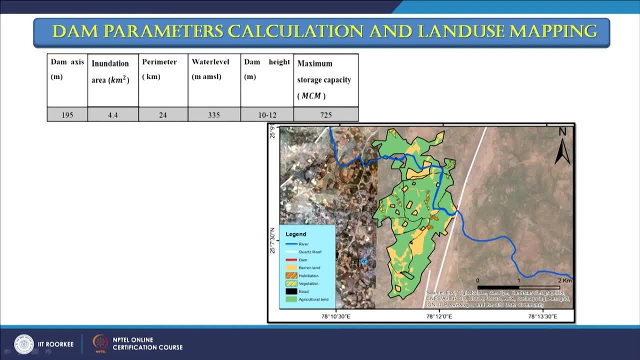 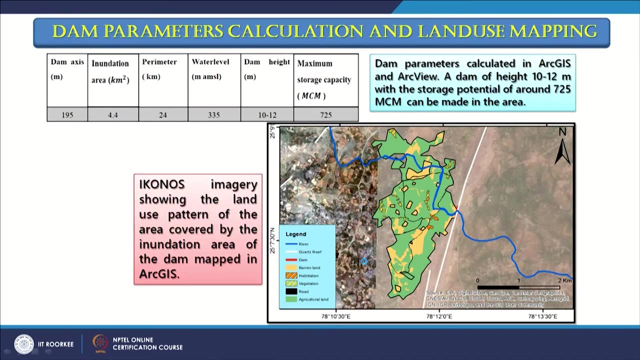 And if you are having revenue record and put this polygon, this is the inundated area of the reservoir, immediately you would know that whose land will be submerged. So if it is acceptable to local people and decision makers, a reservoir can come. In 2 years time it will start providing 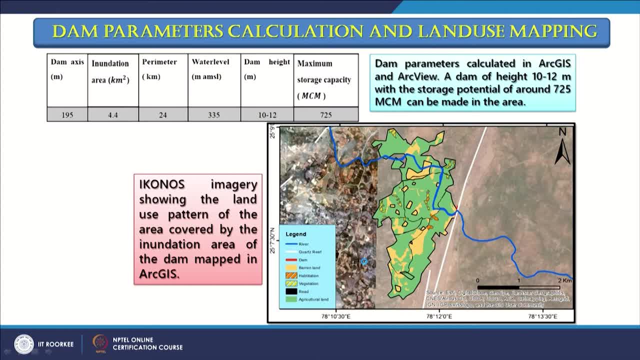 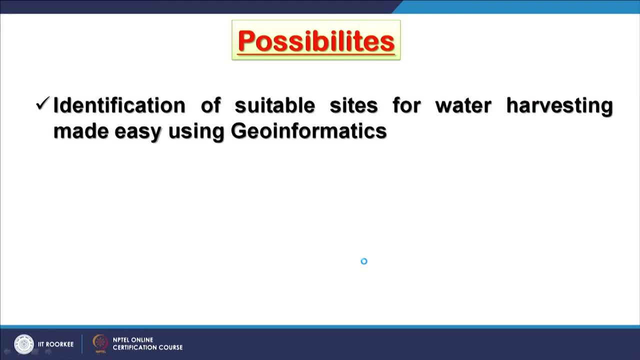 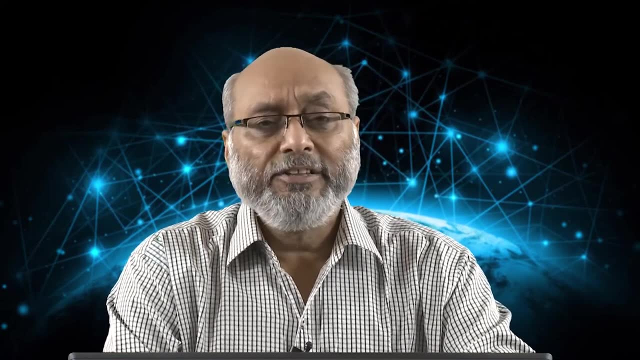 benefits. So what are the possibilities That identification of suitable sites for what are the water harvesting has been made very easy using GIS or geoinformatics technology. Preliminary assessment can be done For detailed project report. obviously things have to be. 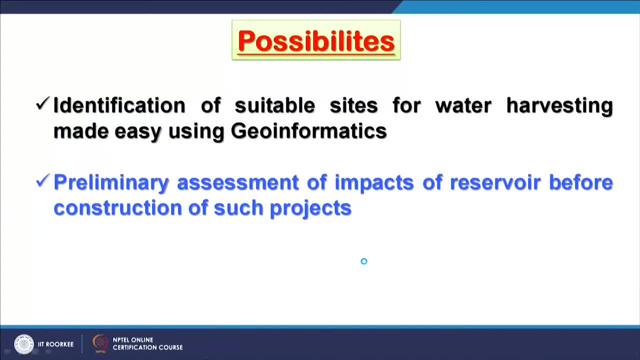 checked on the ground, But feasibility studies can be done very easily and different scenarios, different options can be created for better decisions And simple solutions. This is my whole point of discussion Is what solutions which I am providing are very simple and implement with the local people and 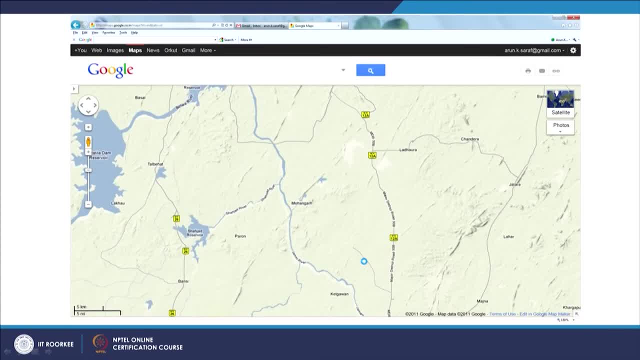 local material. Even if you imply a Google Earth image and have a Google map image, you can see these quartz reefs very clearly on that, Because in the Google map you are also having digital elevation model and that is in the shaded form that is, hill shade, So these things can be. identified Water bodies are also shown there. So this is a very simple solution. But feasibility studies can be done very easily and different scenarios can be made for better decisions. But feasibility studies can be done very easily and different scenarios can be made for better decisions. 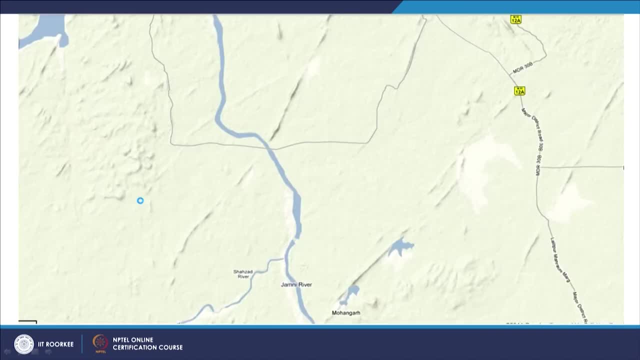 So these things can be identified. Water bodies are also shown there, So data is available. See here, like the quartz reef is running, like this river is moving like this, going like this. Only thing we require to block this one, to make a reservoir like this. 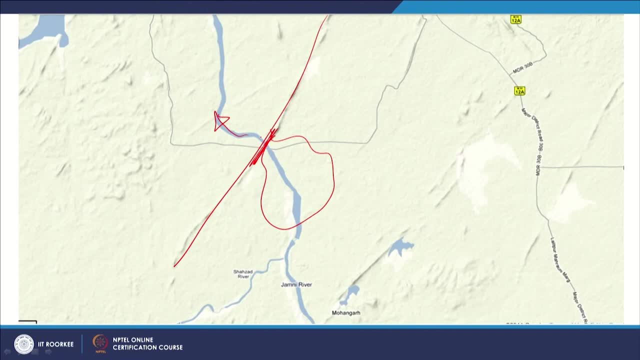 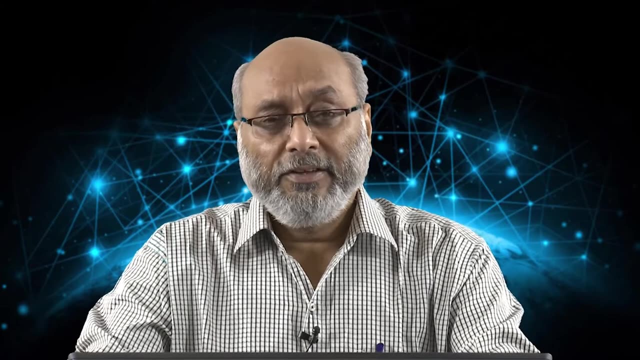 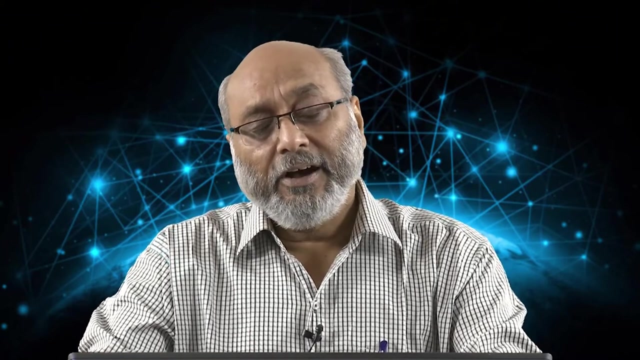 So this is one option. Another thing is how to further assess the situation. You remember that we did a hydrologic modeling in GIS and we created a drainage network. While discussing this surface hydrologic modelling, in the beginning I said there is an assumption. 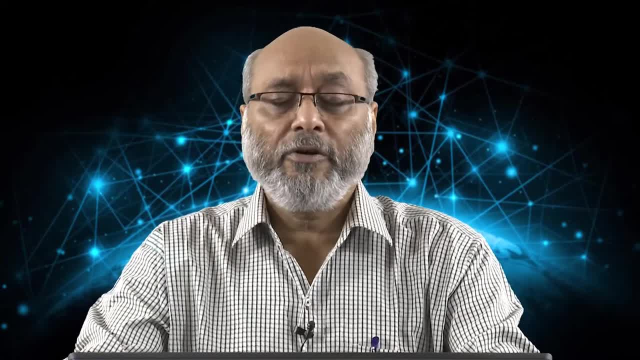 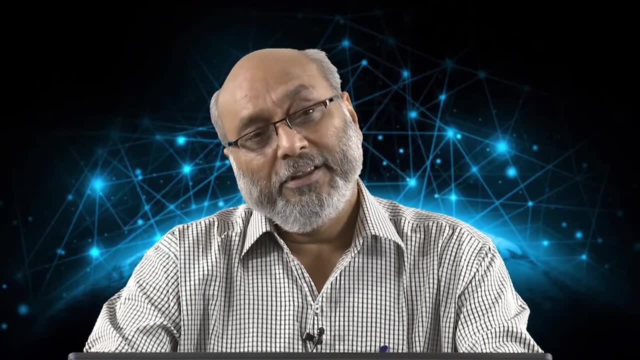 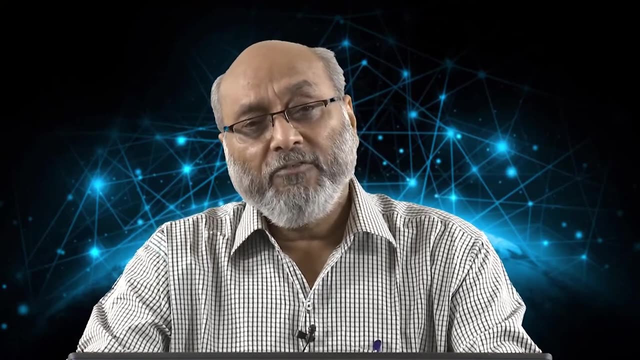 that each drop of water will flow as a surface runoff on the surface. So that assumption is okay. We can exploit even that assumption and can find out just without doing much and just adding one more layer, and can find out which are the areas which will provide. 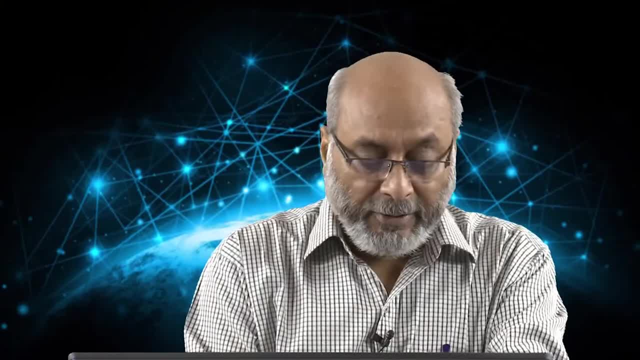 better groundwater recharge. So basically we can find out which are area which will provide better groundwater recharge And these are the areas which will provide better groundwater recharge. So basically we have to compare a simulated drainage versus surveyed drainage. Surveyed drainage: that 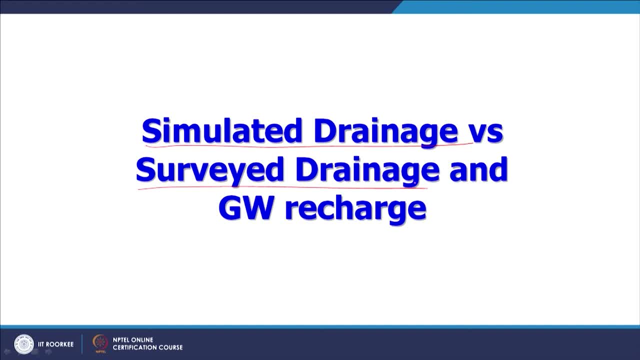 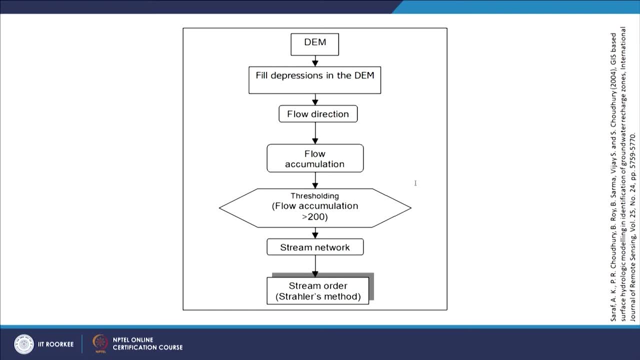 is the real one, which can come from surveyed toposheets And we can get an insight about groundwater recharge. So this part we have already discussed in surface hydrologic modelling: that you use a DEM, you fill it, flow direction, flow accumulation, thresholding, stream network. 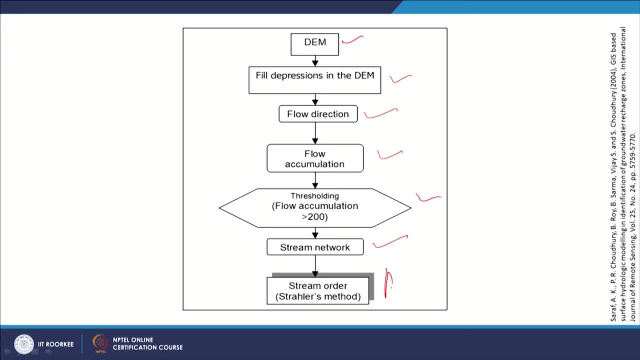 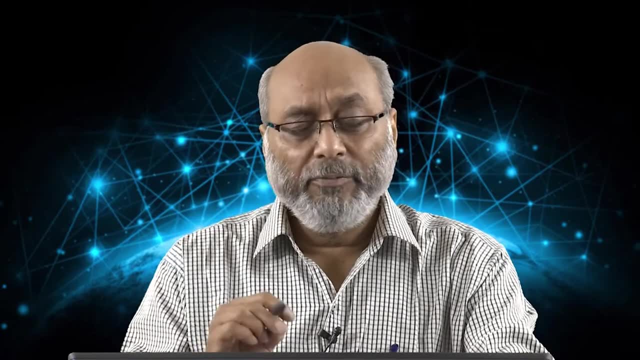 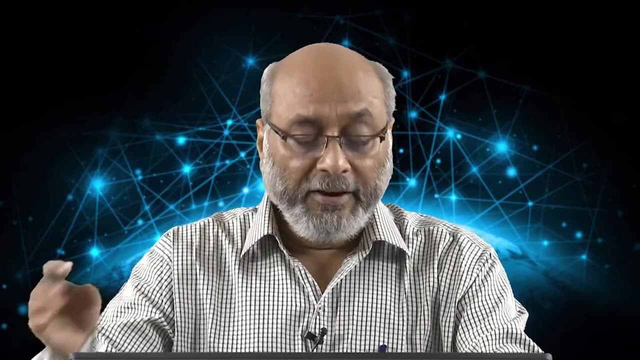 and stream model. So once that is you are having in your system, you also require a surveyed drainage network and that means digitizing whatever the best scale toposheets available for a particular area. And when you overlay these things you would notice that in some parts 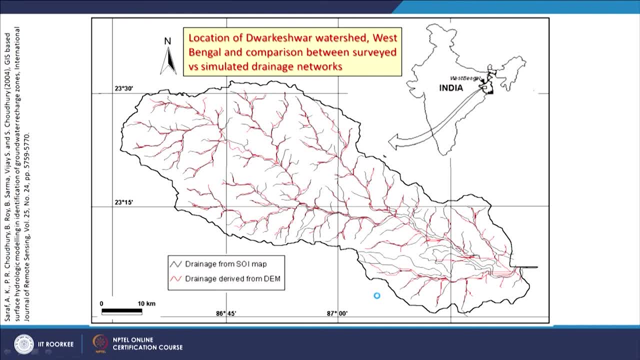 the surveyed drainage and model drainage are almost same. But when you would further observe in some areas, like here in this lower part, that the surveyed drainage and model drainage there is no match, That means that the model drainage is in the assumption that the model drainage and the water has to flow. So there is a deviation and deviation in the 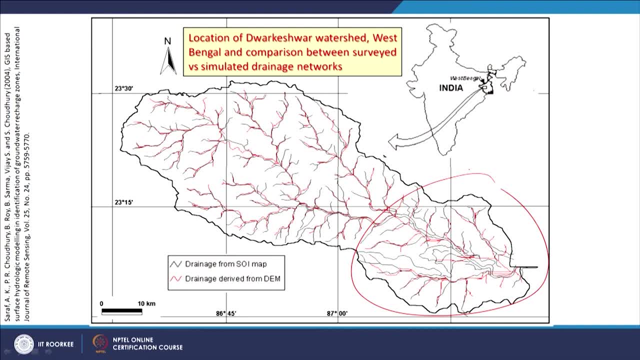 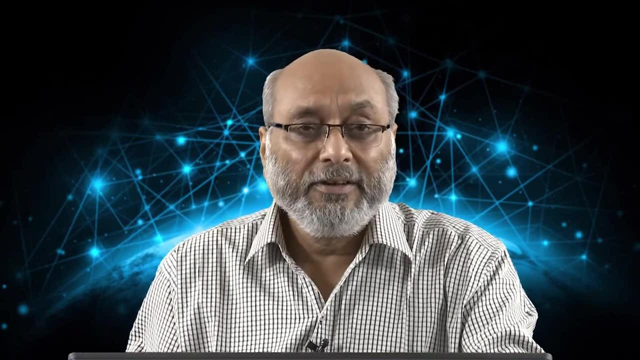 position of the drainage network, Because natural drainage, where whatever the water going towards groundwater regime, that will affect the drainage system. So this mismatch we can exploit and we can say, just comparing these 2 networks, one is modelled, another one is the real one- that wherever, 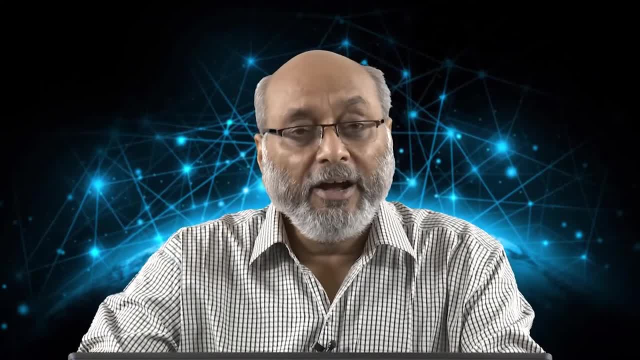 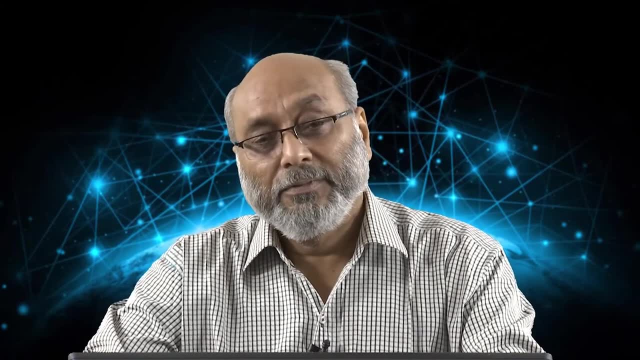 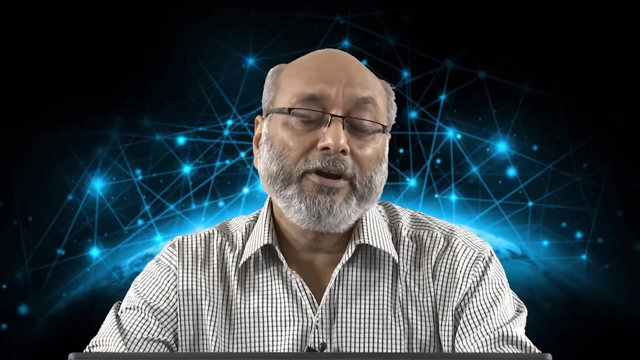 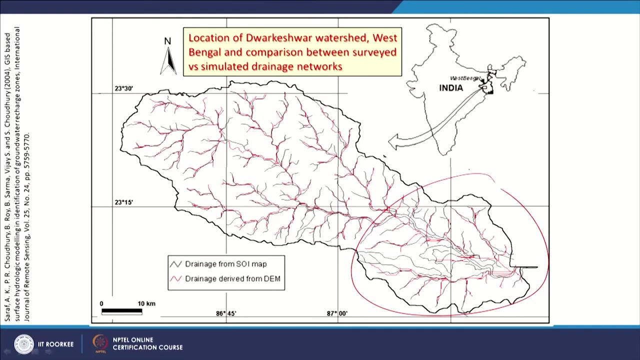 the mismatch, we are having high chance of getting groundwater, and these are the areas where groundwater recharge structure should be constructed, Because that one, the surveyed or real drainage- is not following the modelled drainage concept, And if it is following, that means whenever both are coinciding. that means surveyed drainage and 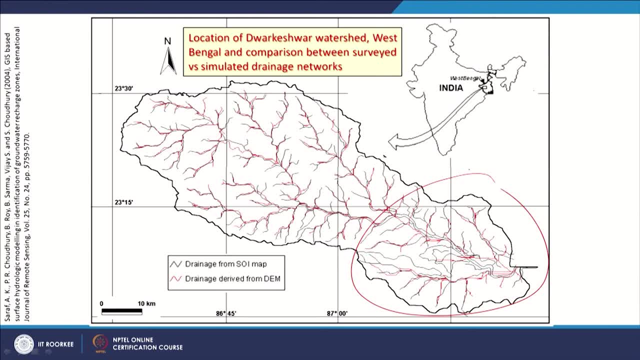 model drainage are same, That means there is no loss of water, assuming that entire watershed is having same evapotranspiration losses. So other losses are to the groundwater. If there is a loss to the groundwater then definitely the model drainage will not follow the surveyed drainage. 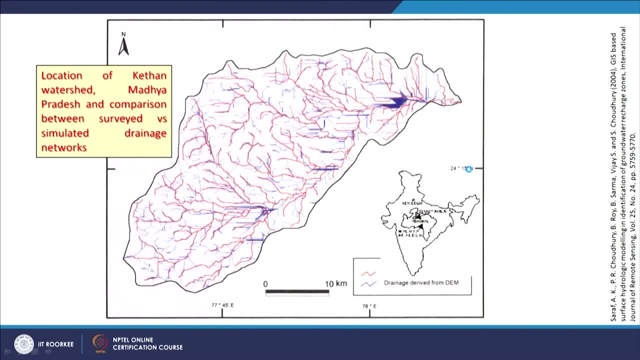 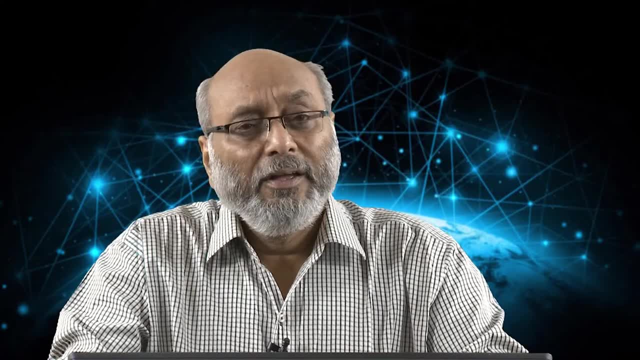 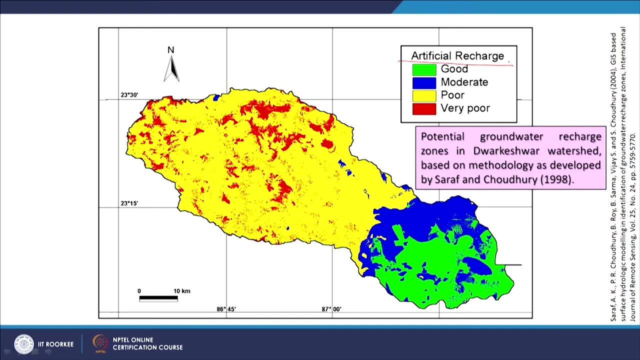 And this mismatch can also be exploited. So very simple technique. One more example of a different area. you can see it works very well. Of course you can find out the areas which are good for artificial recharge groundwater regime, that you can do it quite easily. 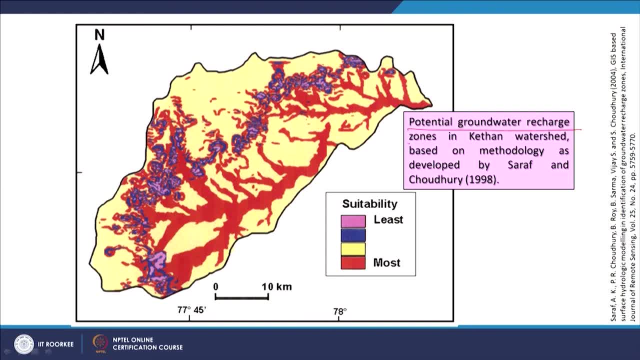 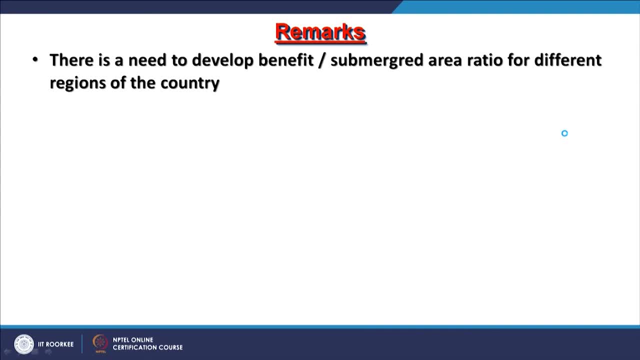 Similarly, you can find out the potential groundwater recharge zones for another basin. So what we see? that by developing this benefit versus submerged area ratio for the different region of the country, if we are having beforehand, we would know that if a structure is created. 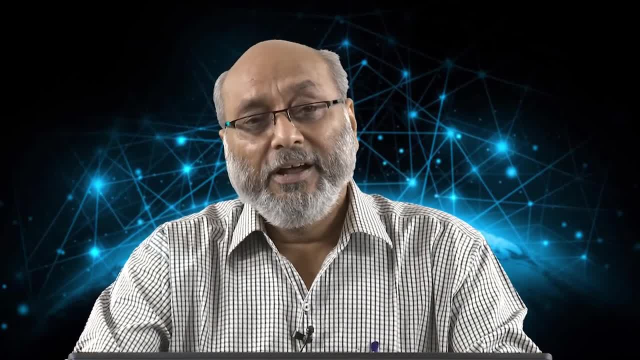 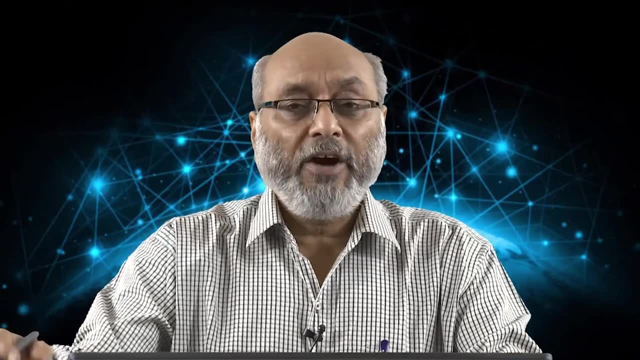 how much benefits in terms of this benefit area I will going to have. What is the return? I am going to, Because decision makers would like to know that. okay, fine, if I construct a reservoir here, I am going to have the return. If I construct a reservoir here, I am going.